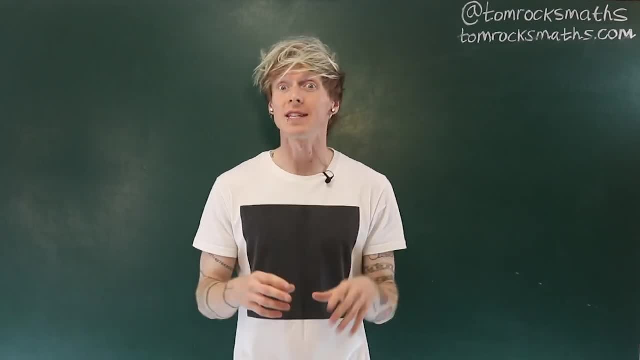 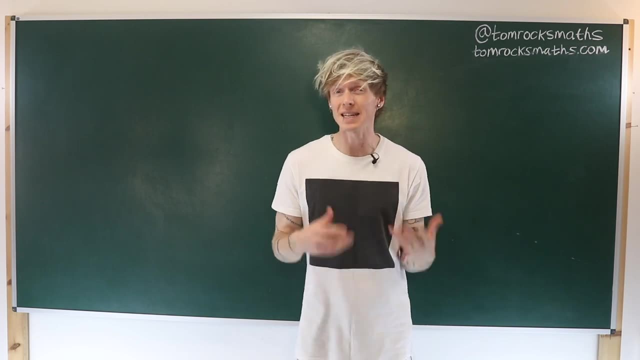 Hello Maths fans, Dr Tom Crawford, here at the University of Oxford, and today we're looking at how to calculate the determinant of a matrix. So far in the linear algebra series, we've looked at solving systems of linear equations and calculating the inverse of a matrix. Now what? 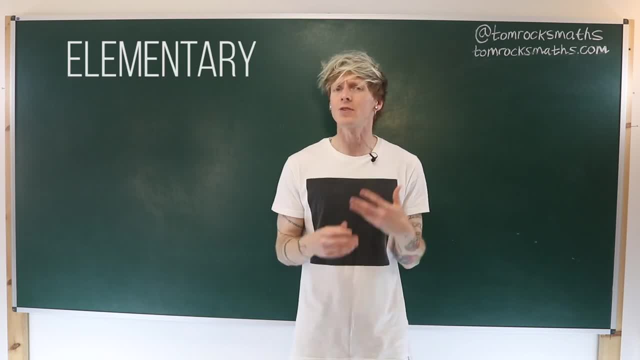 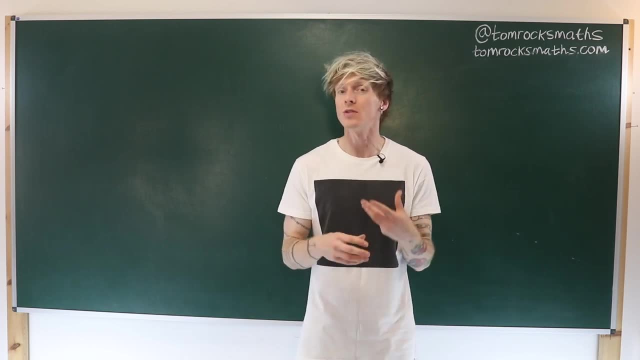 both of these topics have in common is the use of elementary row operations, or EROs. When looking at determinants, we can once again use EROs to simplify our calculations, and that is exactly what we'll be doing in part two of this video. In part one, we'll look at the 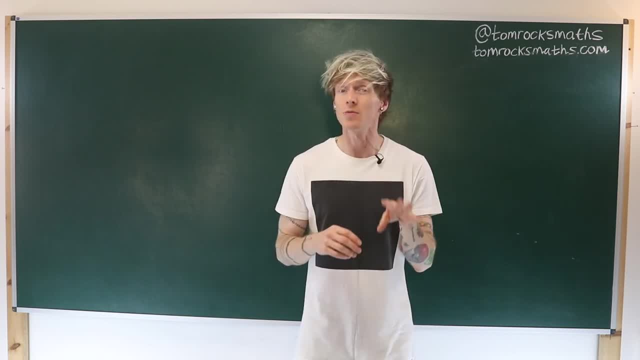 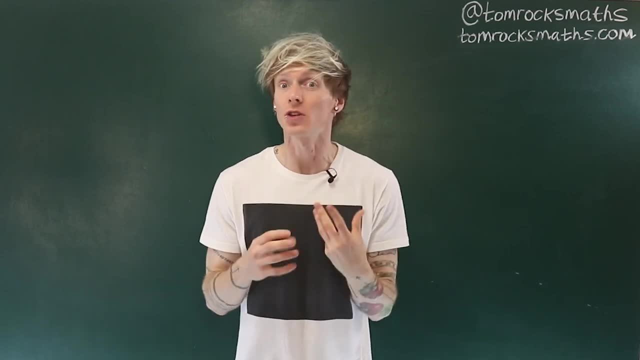 theory behind the general formulae for determinants of a two by two and three by three matrix. As usual, I'll be going through some worked examples to help to build your understanding. and don't forget: you can sign up for a 30-day free trial with ProPrep, where you can. 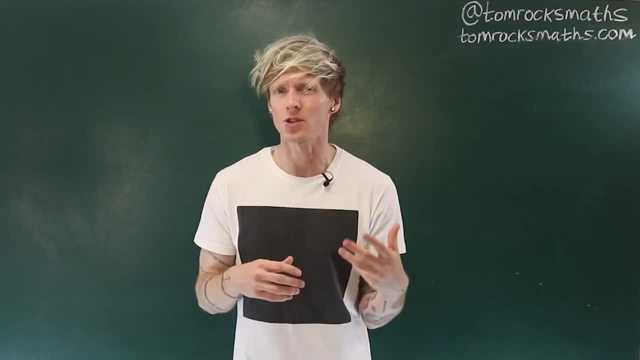 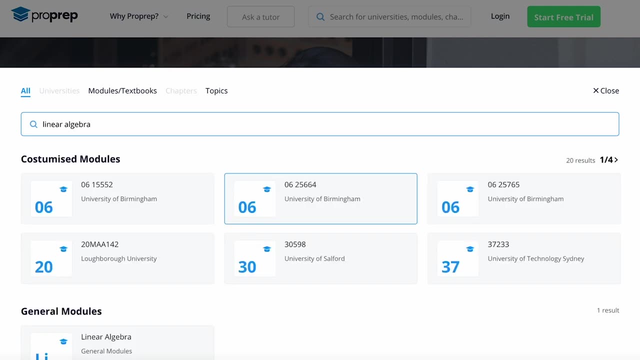 actually use EROs to simplify your calculations. If you're interested in learning more about EROs, you can access many more examples, each with a video solution. ProPrep is an online resource that provides customised tutorials for students looking to improve their skills in STEM-based. 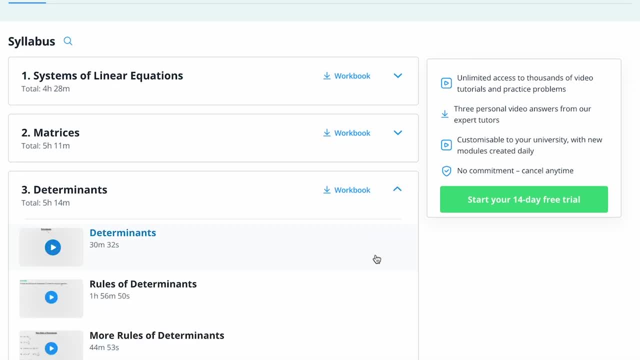 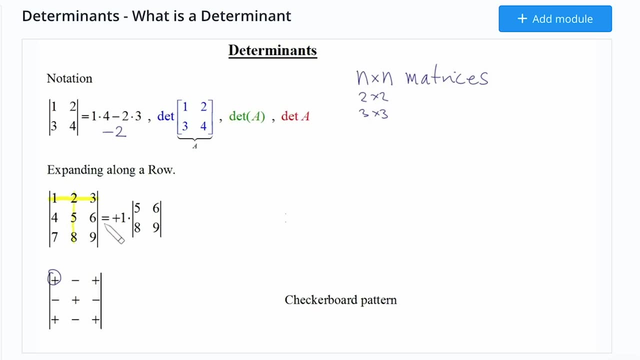 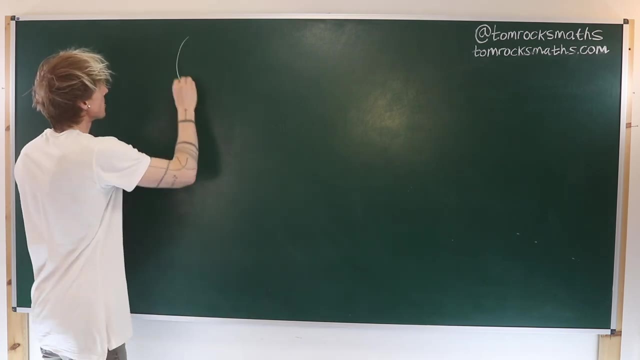 subjects. All of the ProPrep exercises are available via the links in the video description and you can access the videos by signing up for a free trial using the link below. For our first example, let's look at a general two by two matrix. So something of the form. 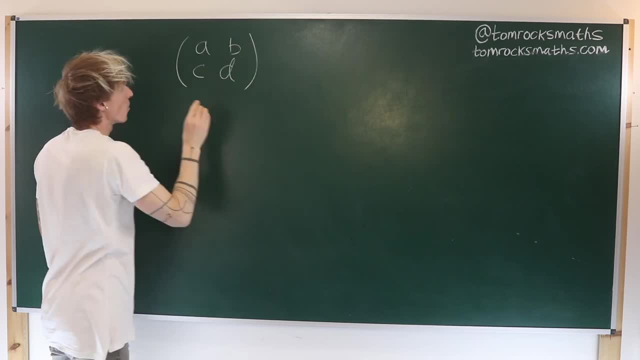 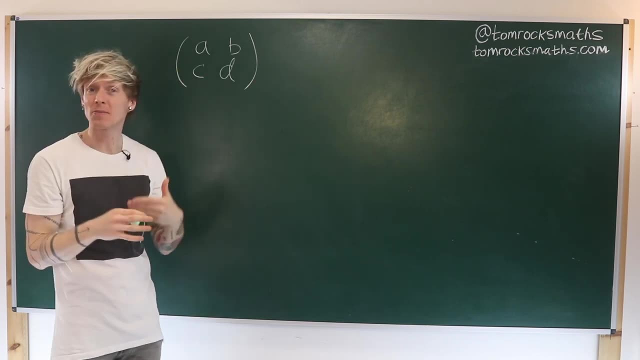 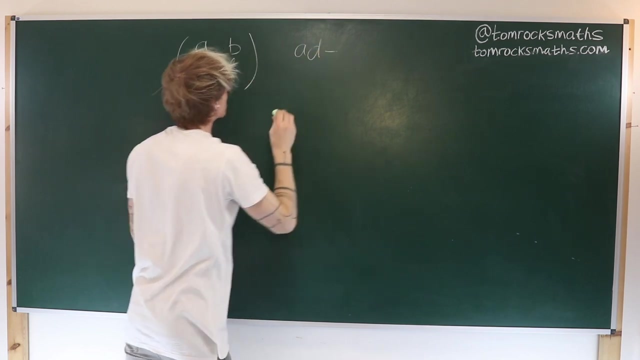 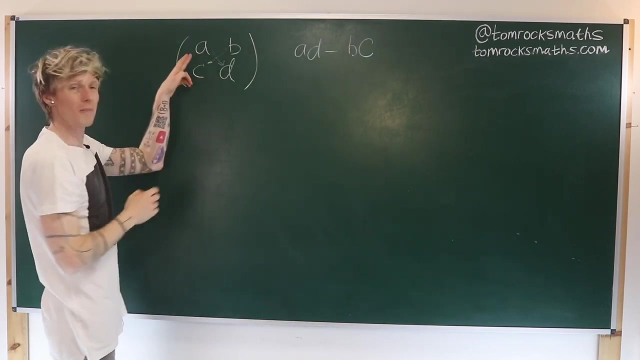 a, b, c, d, where these entries, of course, could be any number. Now we define the determinant of this two by two matrix to be a times d minus b times c. So what we're doing is the top left multiplied by the bottom right, and then you subtract the top right. 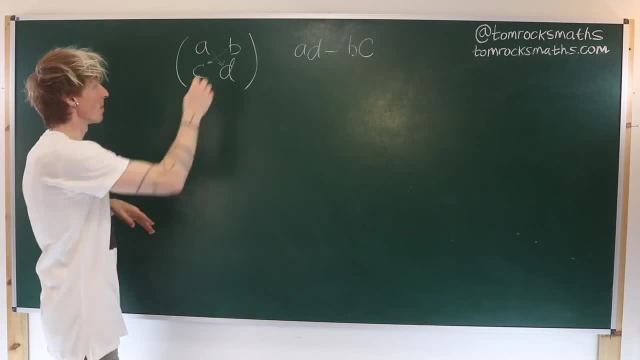 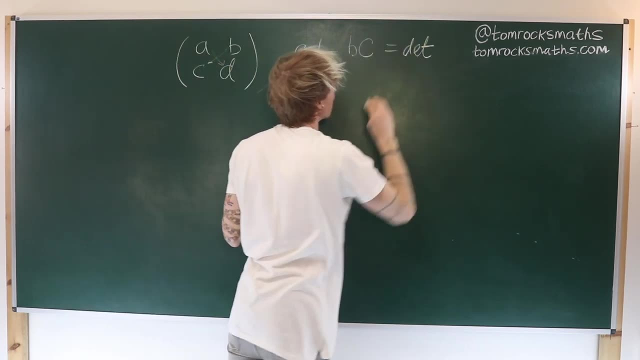 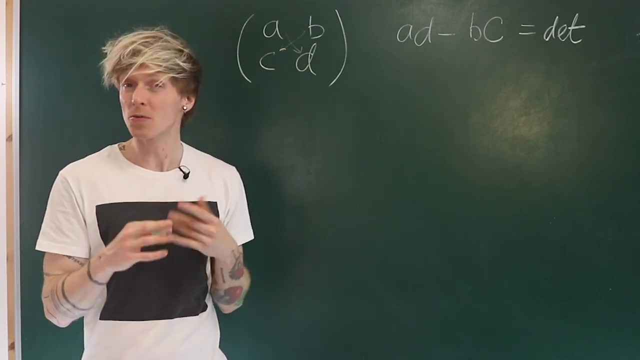 multiplied by the bottom left. So if you just remember, for this matrix a, b, c, d, the determinant is equal to a d minus b, c. Now to understand exactly why this is how we calculate a two by two determinant is quite advanced. So I teach this in the linear algebra two course. 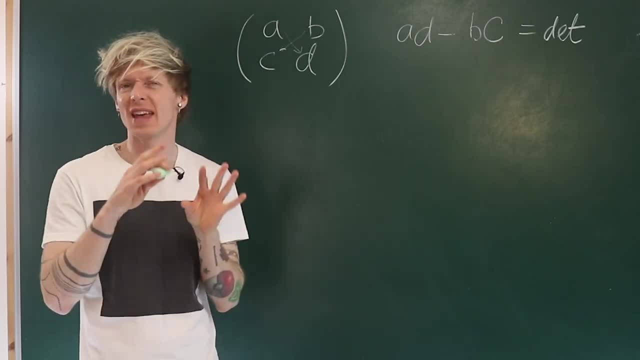 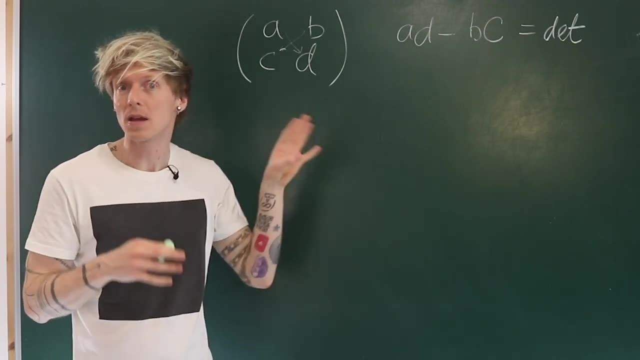 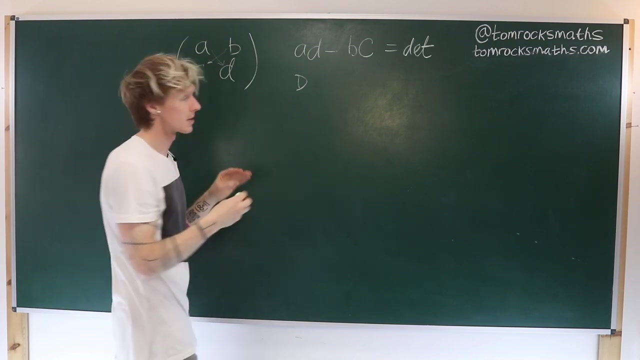 here at Oxford to my first year students, but this is taught in their second term. However, I'll go through the basic idea, just so you have a flavour of where this comes from. We start by considering a general function, d, and this is, of course, going to be our determinant. 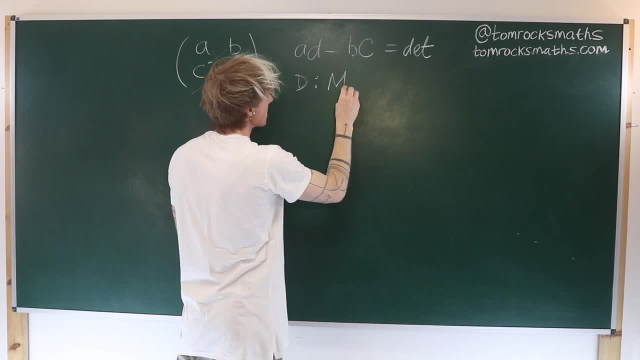 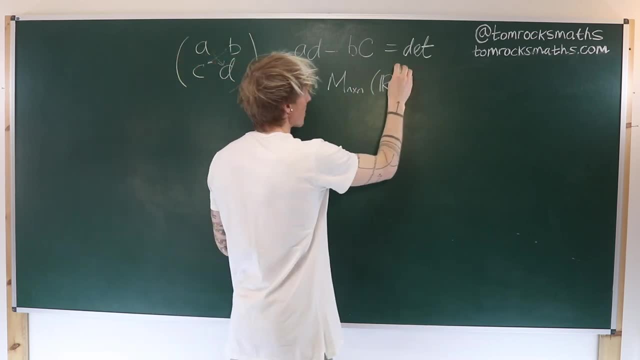 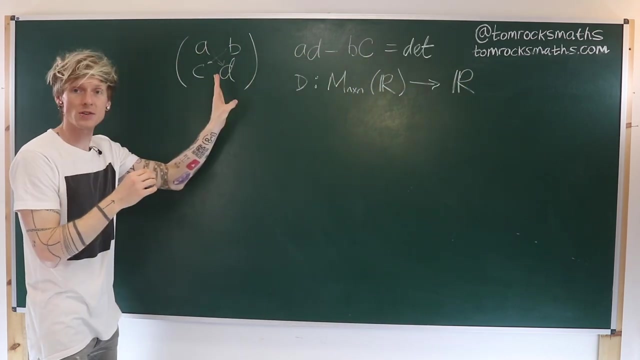 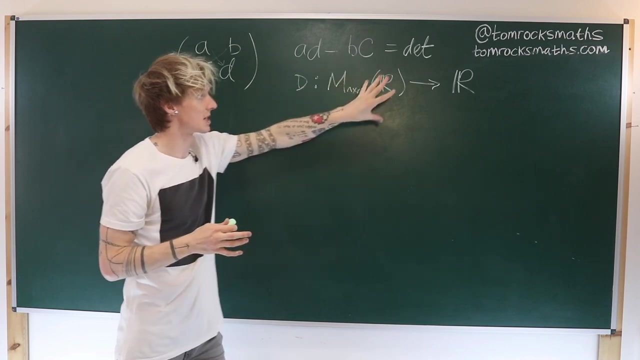 And we want this function to map from the n by n matrices and just to make it easier here, we'll just consider real entries. So it's going to map from a matrix to give us a real number And we output this scalar: a d minus b, c. So this is clearly mapping from matrices to the. 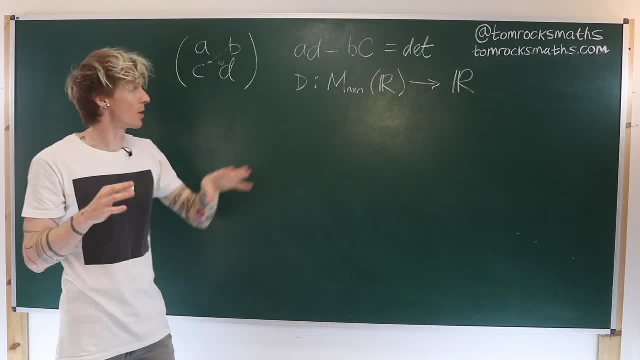 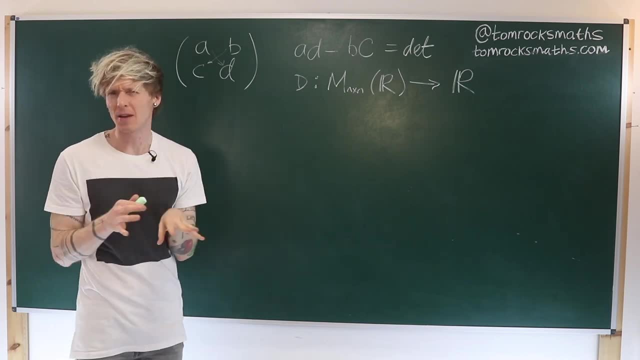 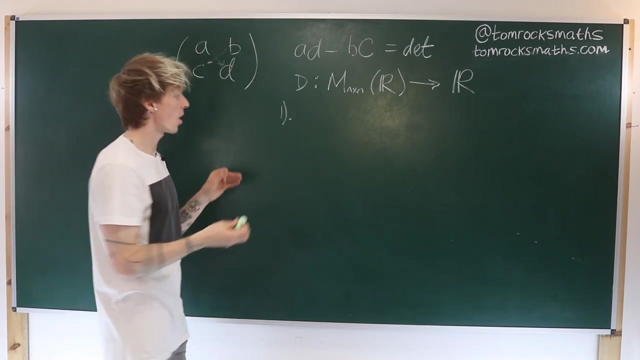 real numbers, where here n is two. Now we want to look for a general function of this form such that it satisfies three specific properties. So the first property that it needs to have is that if we swap the order of two rows- So swapping two rows- we're going to get a. 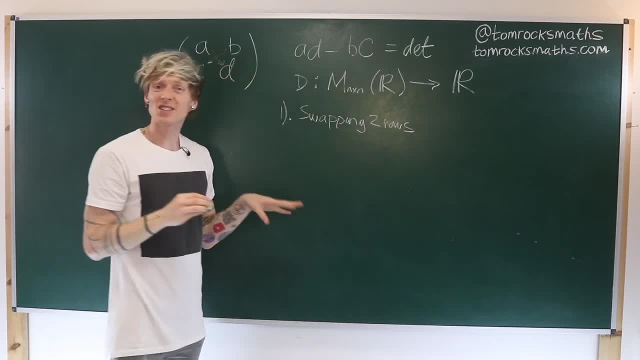 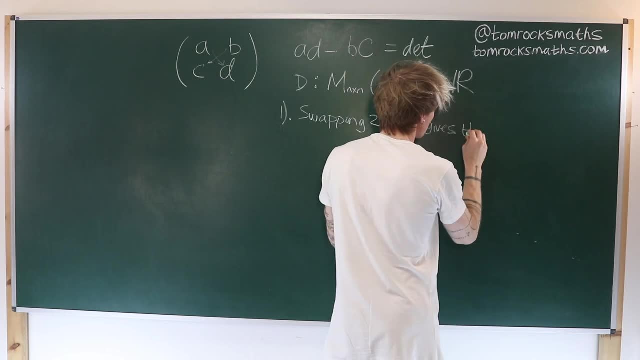 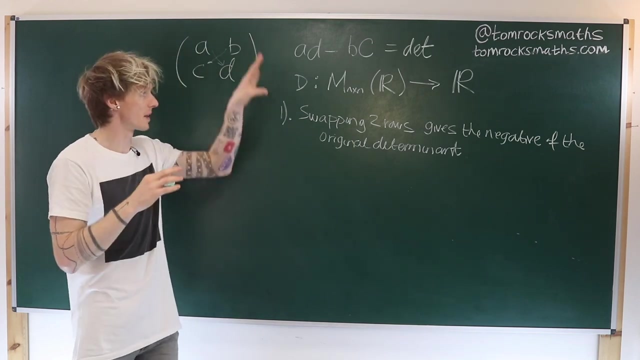 negative of the original answer. So swapping two rows in our matrix should actually give the negative of the original answer. So swapping two rows gives the negative of the original answer for the determinant. So that's going to be our first property, that we want this general function d our determinant. 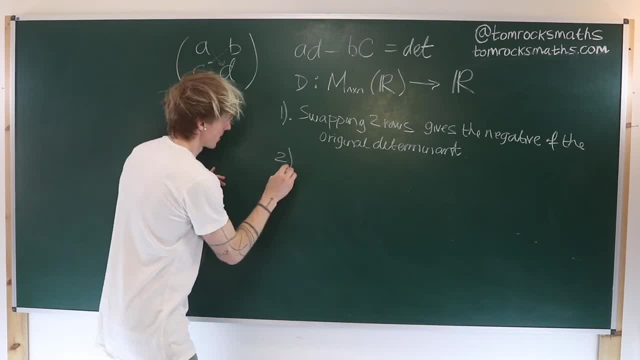 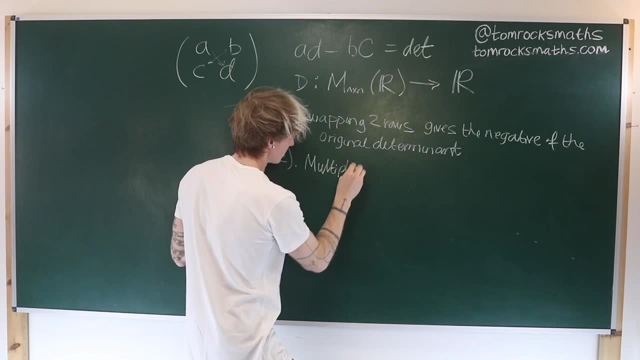 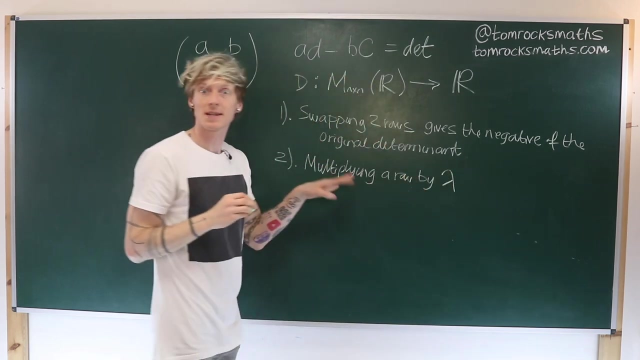 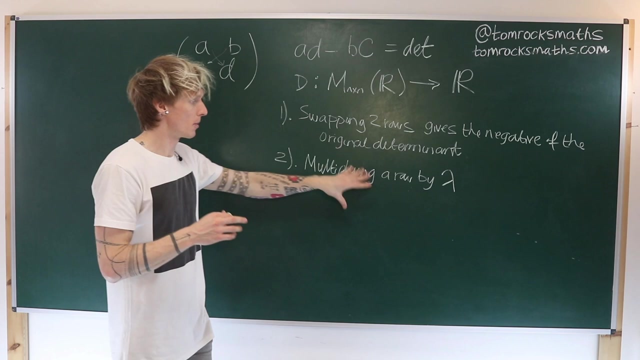 to satisfy. Now, the second property that we want it to satisfy is to say that multiplying by a scalar, or multiplying a row by a scalar, by lambda representing our scalar, then that multiplies the answer by the same scalar. So notice, we're not multiplying the whole. 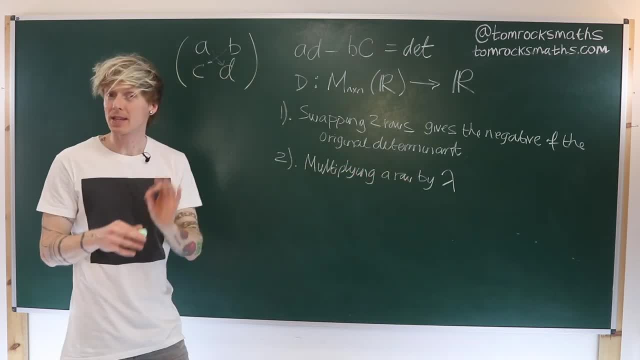 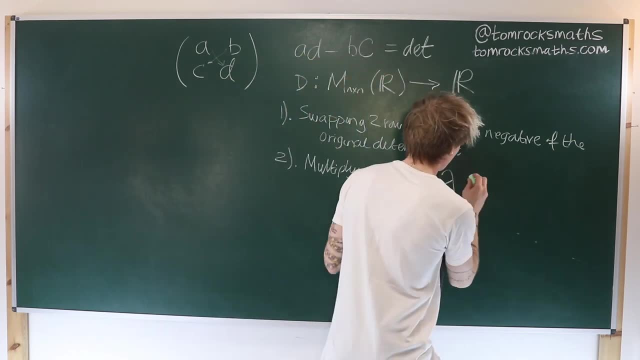 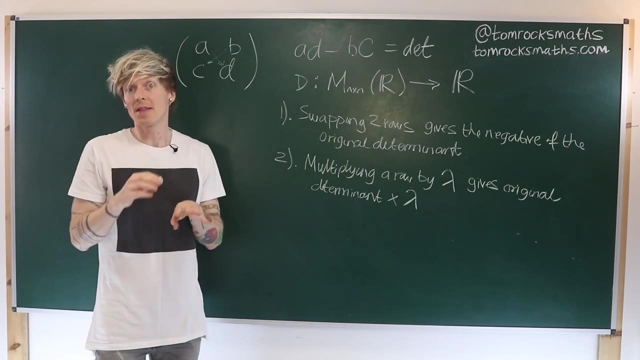 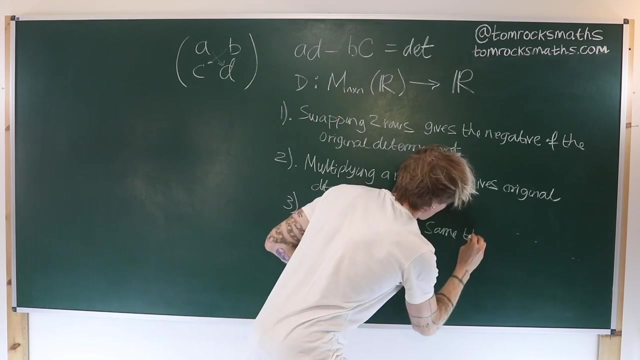 matrix by this scalar. just multiplying a single row gives an answer that has lambda in front of it. So multiplying a row by lambda gives original answer for the determinant times lambda. And then the third and final property is that if we have two rows of the same, then the determinant should be zero. 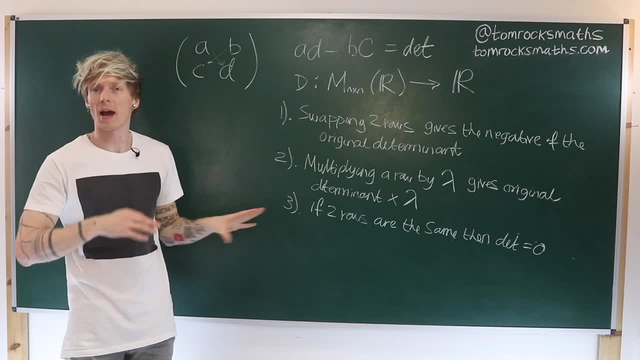 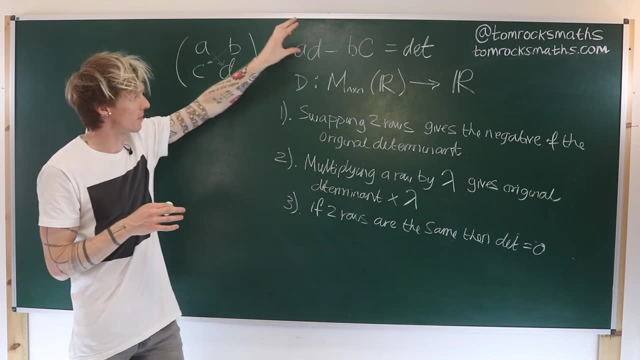 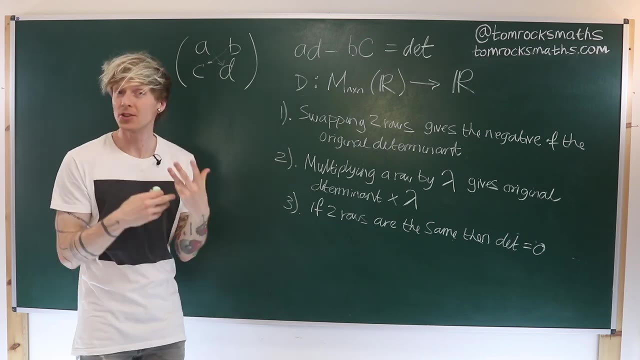 So with these three specific properties- and I'm aware this is quite abstract and quite general at this stage- but if we define a function d from the matrices to the real numbers, such that these three properties are satisfied, then you can show that the determinant is: 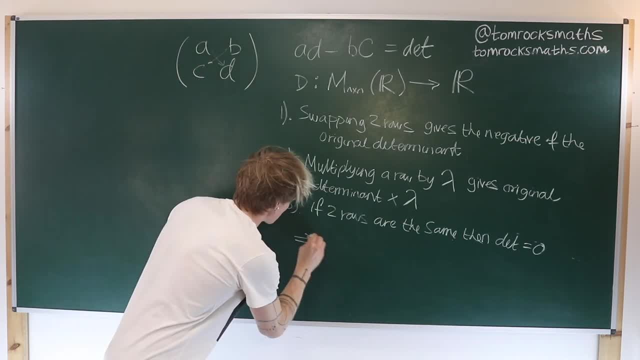 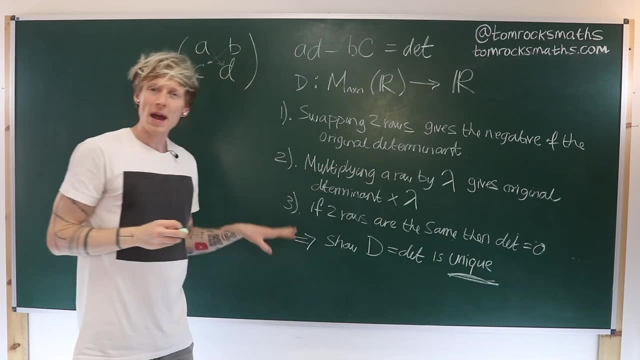 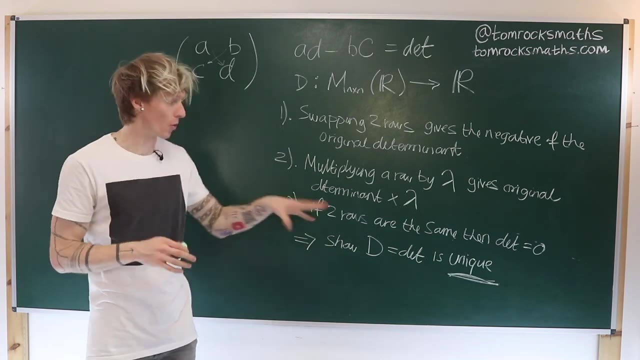 in fact, unique. So, given these three properties, you can show that this function d, which is going to be the determinant function, is unique. Now, where this is really helpful is as follows: If we can write down a candidate for this function, So if we can write down a function, 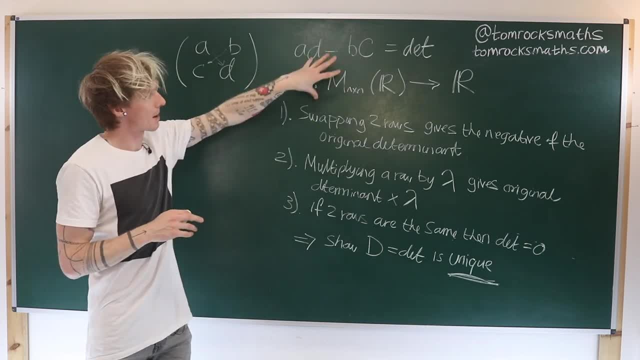 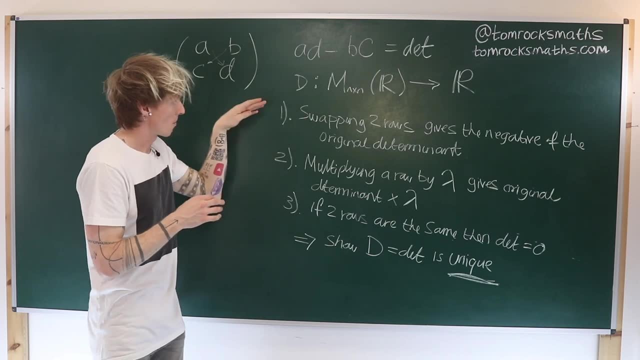 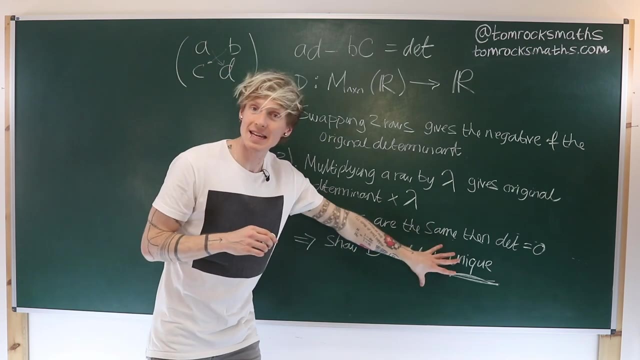 d, which we'll call the debt, such that it maps from a square matrix to a scalar, to a real number. if we can write something down such that properties 1,, 2, and 3 are all satisfied, then because it's possible to show that anything satisfying this is unique. there is only one such. 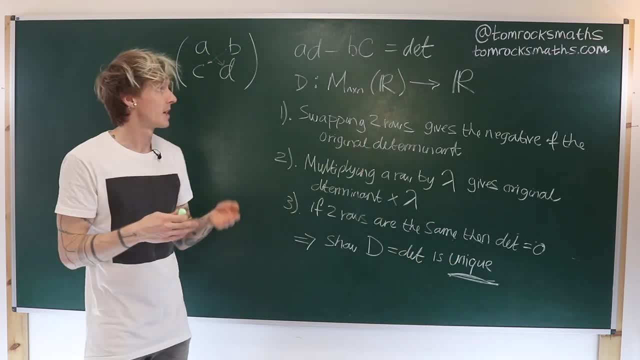 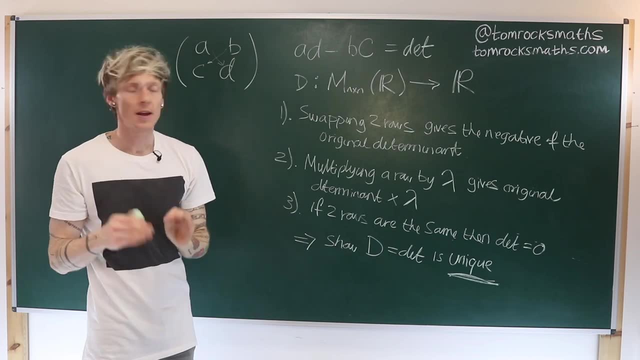 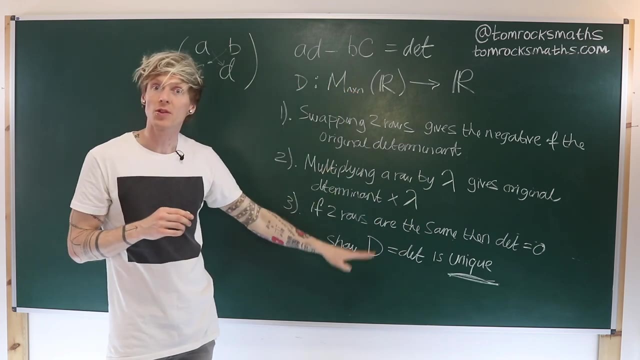 function doing this. if we can come up with that, maybe try something like this- then this must be the determinant, because we're saying: all determinants satisfy these three rules. however, that allows us to show that the determinant itself is a unique function. 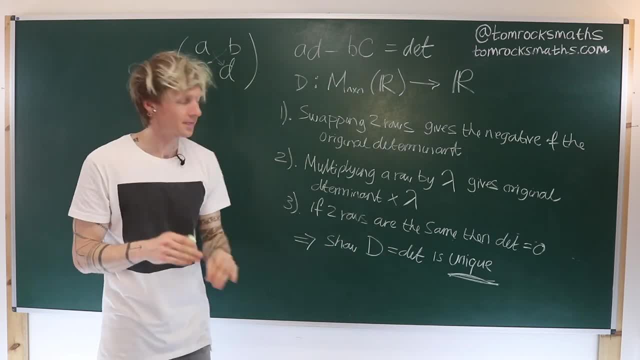 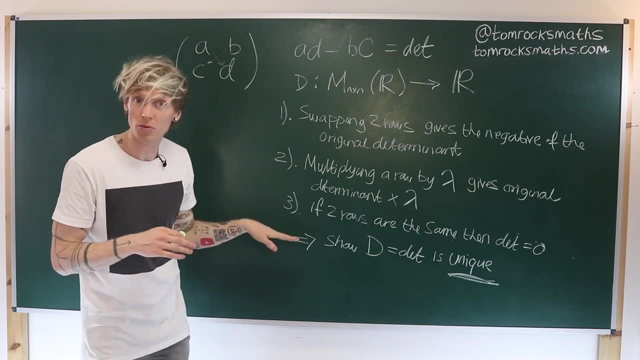 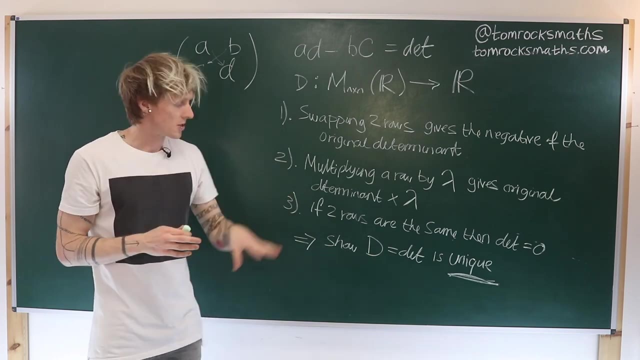 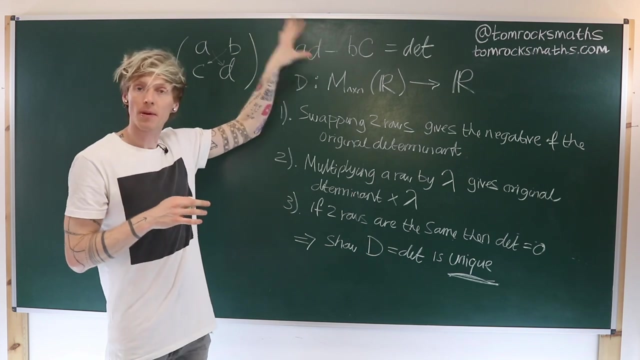 these properties define a unique function. so if we can then write down a candidate to be that function and show that it satisfies these three rules, then we have in fact found the unique determinant, because only one exists. so uniqueness here is really really powerful in allowing us to show that this is indeed the determinant function. 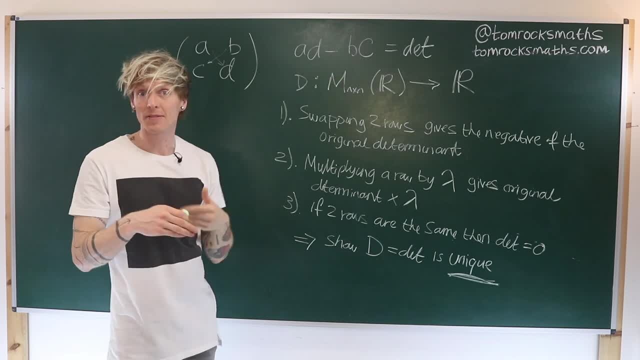 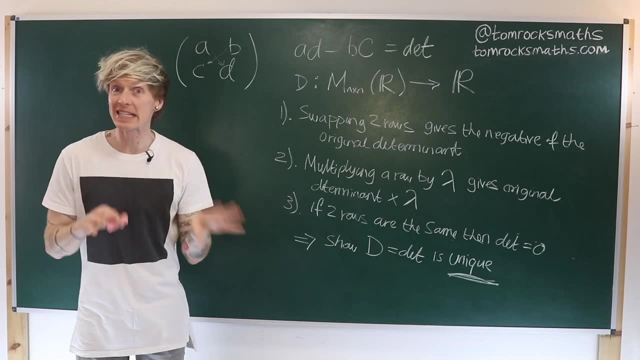 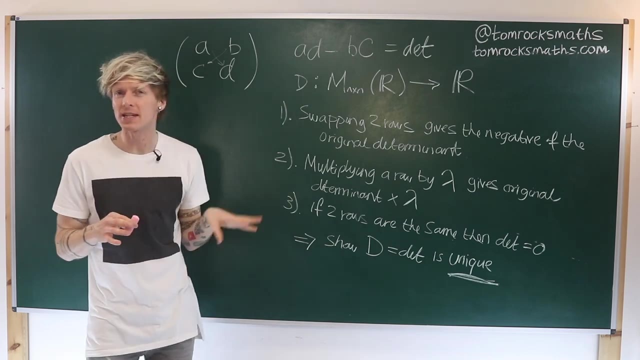 for a two by two matrix. so to show that, all we have to do is show that this function satisfies these three rules. Now, just as an aside, some of you may be looking at these three properties and thinking that they look quite familiar, and you'd be right. they're very. 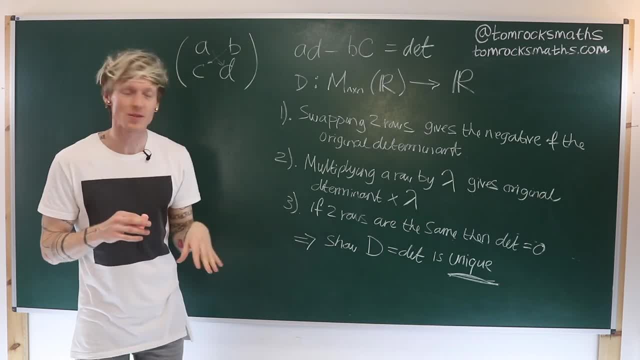 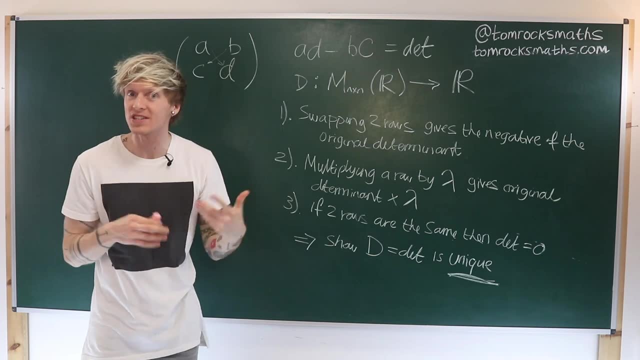 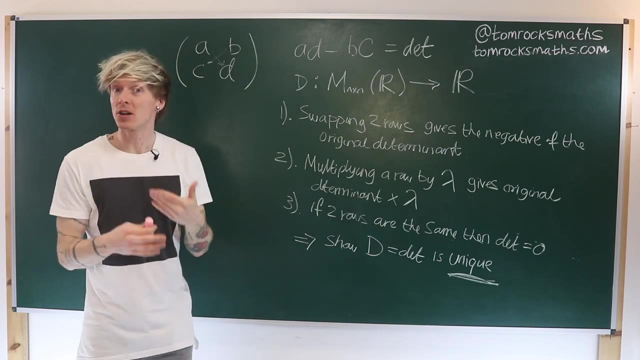 similar to elementary row operations. We're talking about multiplying rows by scalars, we're talking about repeated rows, which we saw in the systems of linear equations video, and we're also talking about swapping two rows. So we will see in part two of this video. 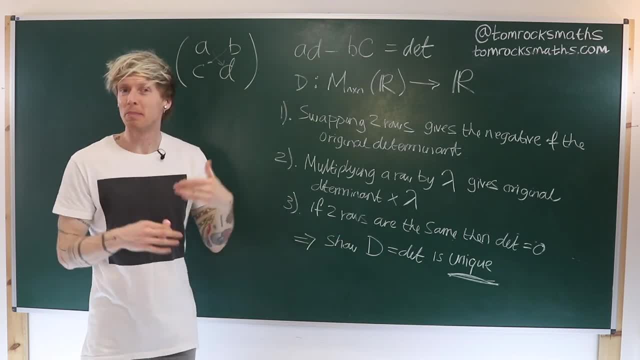 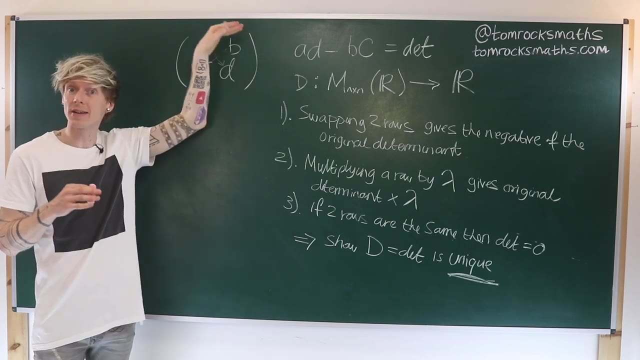 exactly why these properties are so important: because we can use EROs to simplify our calculations and make calculating determinants much easier. But more on that in part two. So now let's check that our function or our definition of a 2x2 determinant. 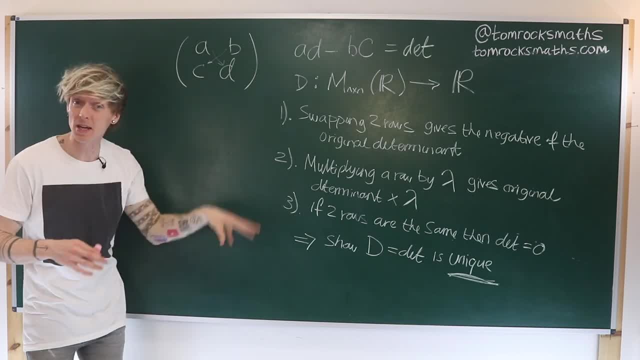 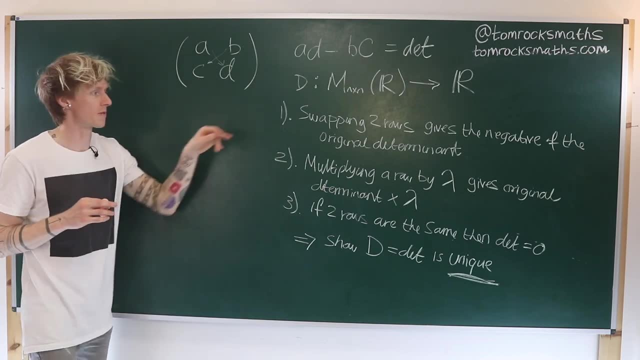 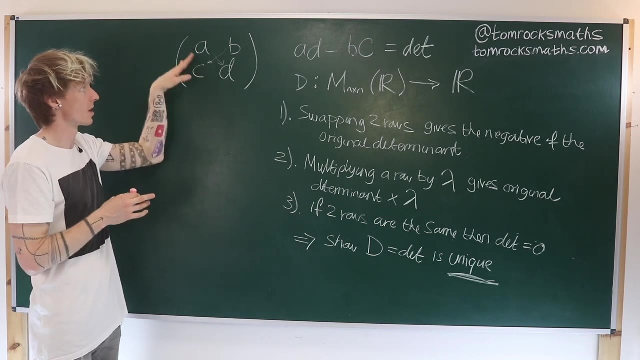 satisfies these three rules Because, remember, if it does, then we have the unique determinant for a 2x2 matrix. So the first property says if we swap two rows we should get the negative of the original determinant. So the original determinant of 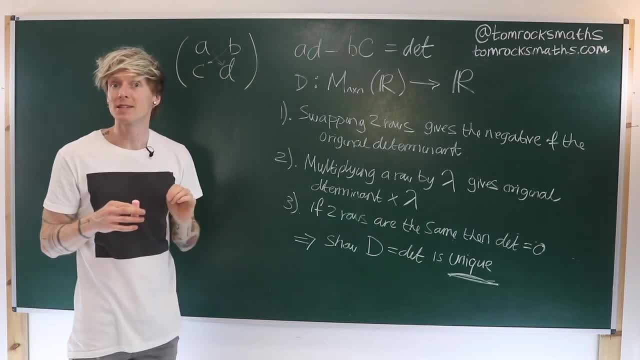 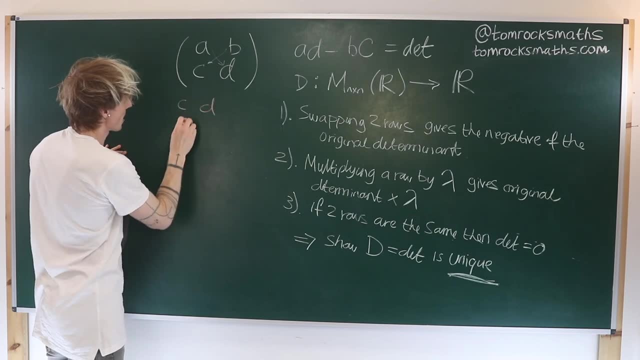 8x2 is the negative of the original determinant of 8x2.. So if we swap two rows, so that means putting C and D on top and then A and B on the bottom. So we only have two rows. so I just have to swap those two. 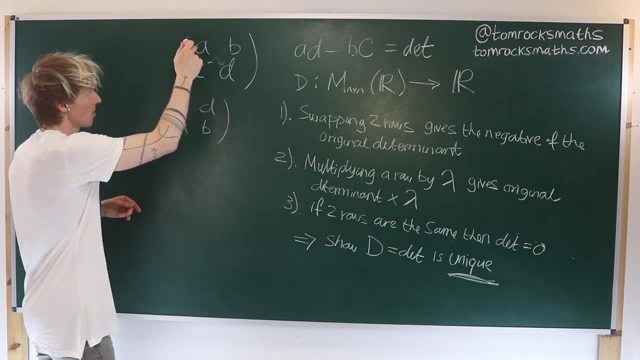 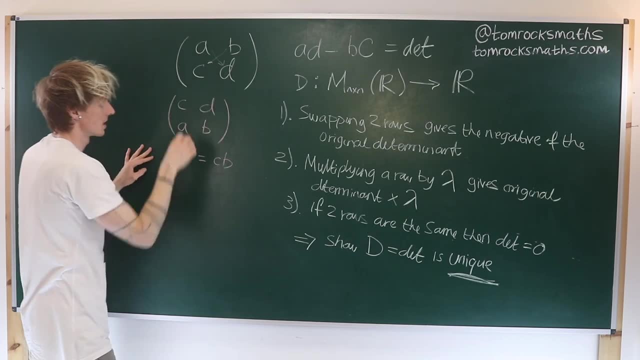 And now, if we use our same definition, so we take top left times, bottom right, so we can say here the determinant of this is CB minus DA. But this is very important because if we swap two rows then we get the negative of the original. 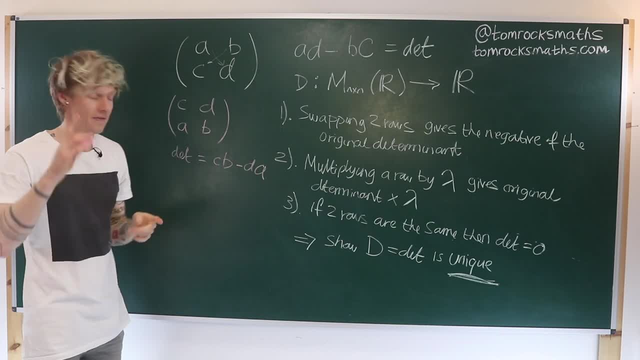 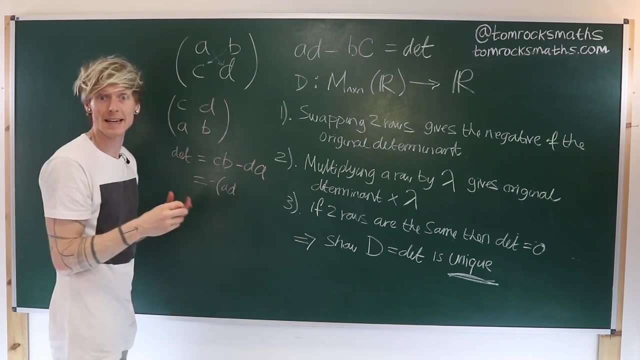 determinant. So this is very similar to the original determinant And in fact it's exactly what we want, Because if I take a minus out the front, then I can write that as AD. DA is the same as AD when you're working with scalars, real numbers, And then we've got minus BC. 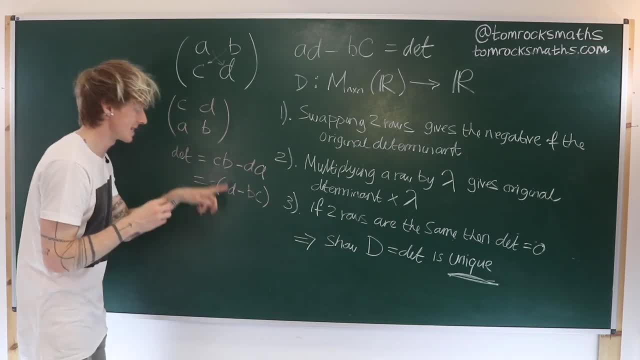 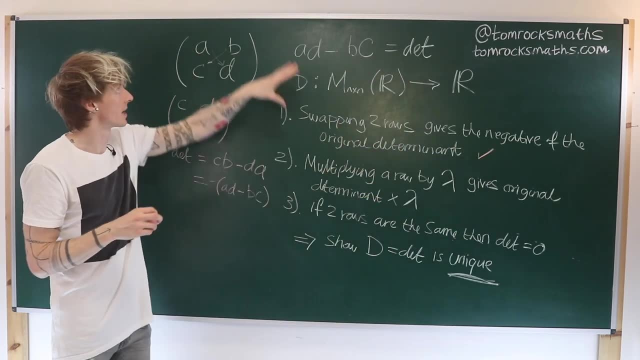 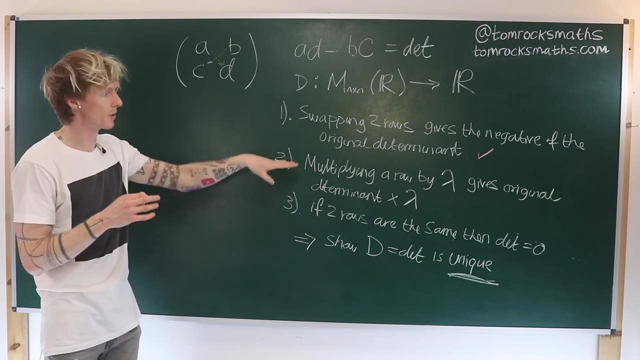 So the answer here, having swapped two rows, is indeed the negative of the original determinant. So this is satisfied. Property 1 is satisfied by this definition for a 2 by 2 matrix determinant. Now for the second property. we need to multiply a single row. 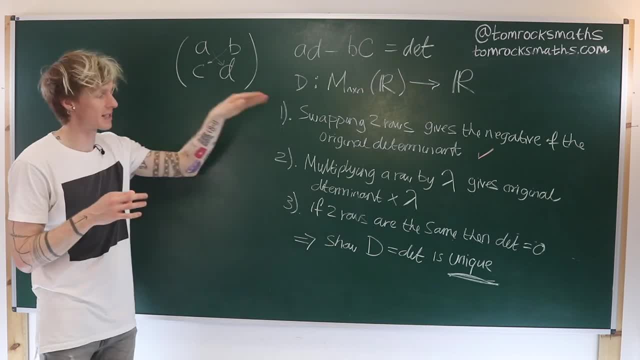 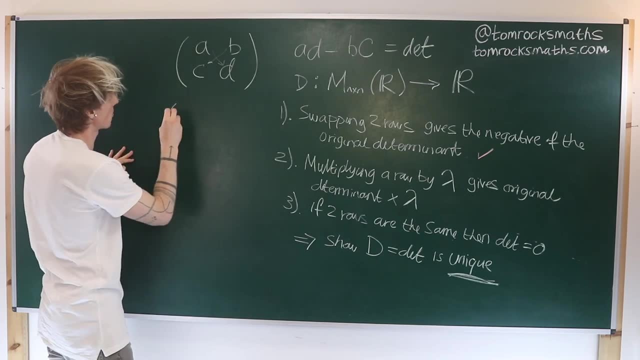 in our original matrix And we should get the same scalar. we'll call it lambda multiplying, our determinant. So let's try that. So let's just multiply the top row and we'll have lambda A, lambda B, and then we've got C, and then we've got D. 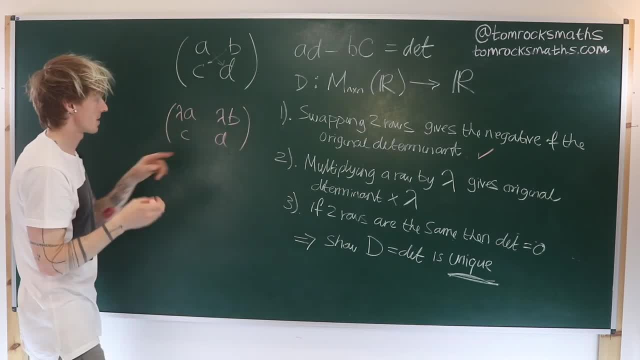 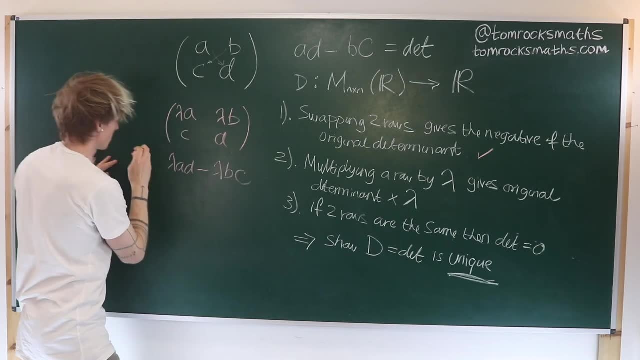 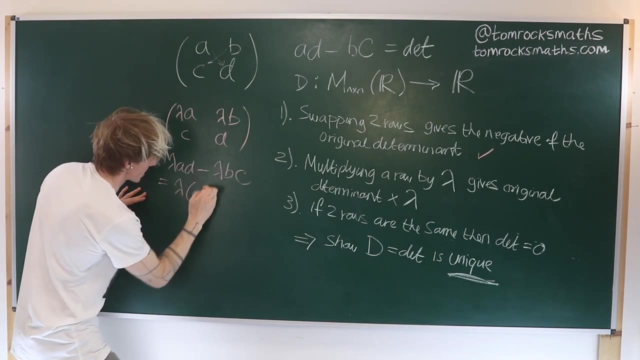 So now we calculate the determinant in the same way: Top left times, bottom right. so that's lambda minus lambda b c. so that's our depth, but of course we can factor out that lambda, and it's lambda ad minus b c. 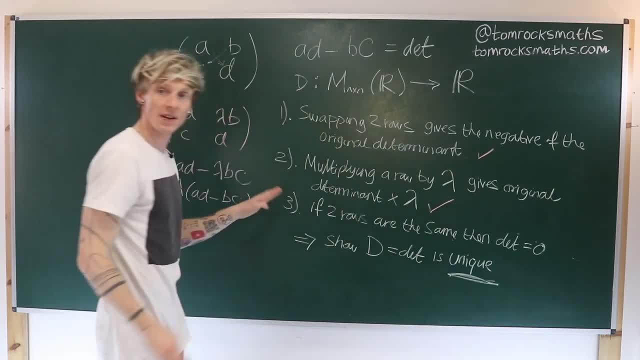 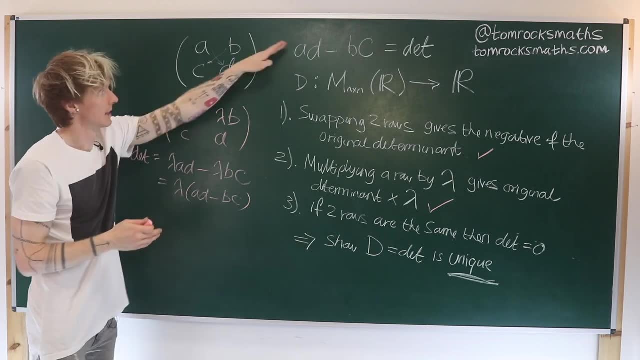 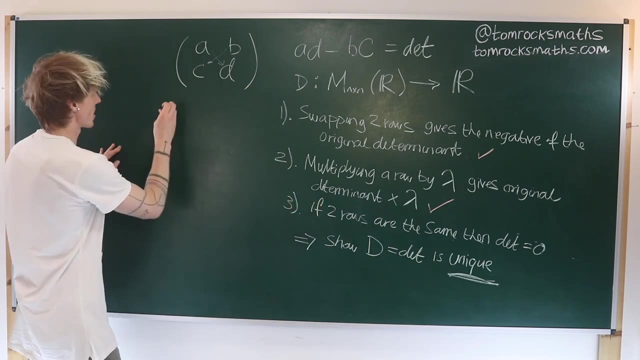 So again, property 2 is satisfied. we multiply a single row in our matrix by lambda and it multiplies the whole determinant by the same scalar, as we can see here. For the third property we need a repeated row in our matrix. So let's just write out 2 times the first row, so ab and ab. 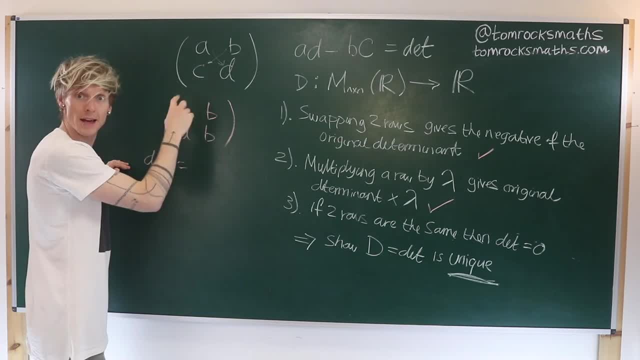 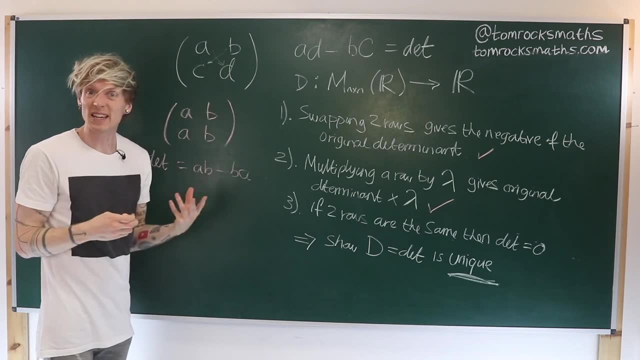 Then if we calculate the determinant again, it's top left times, bottom right. so that's ab minus ba. But once again a and b are scalars, they're real numbers. so this is just 0.. So property 3 is also satisfied. 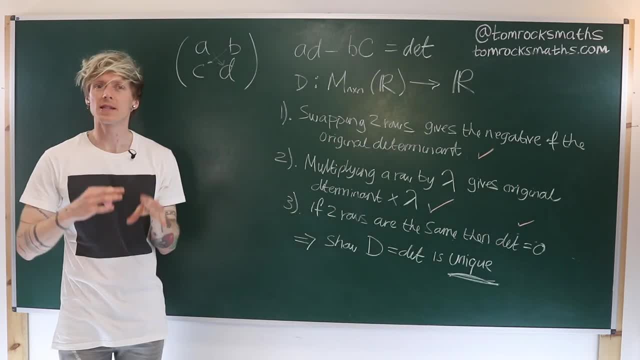 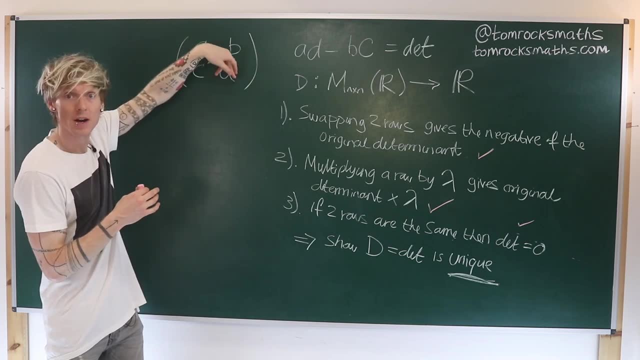 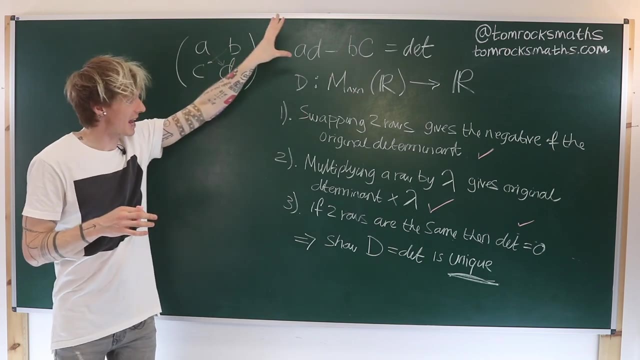 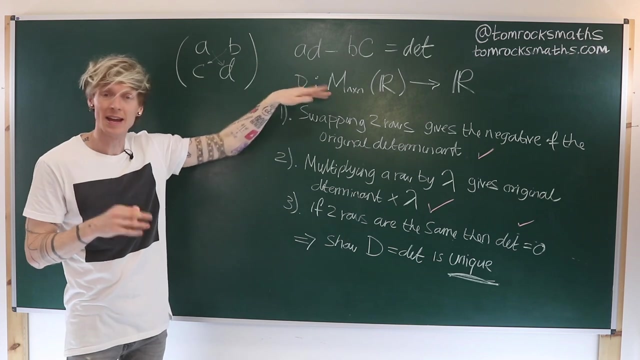 So, in summary, what all does this mean? What all of this means is that the function we have here- ad minus b, c, ie top left times, bottom right minus top right times, bottom left- this function for a 2x2 determinant satisfies all three properties, so it satisfies everything required to be a determinant function. 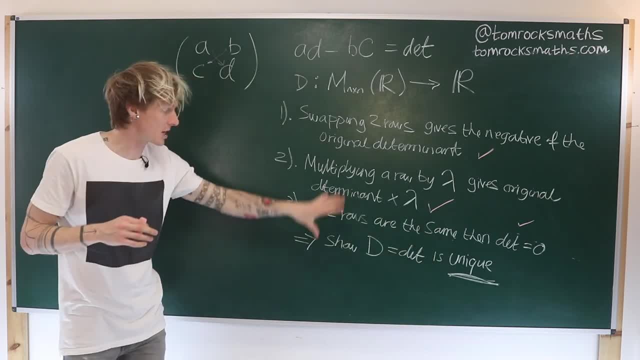 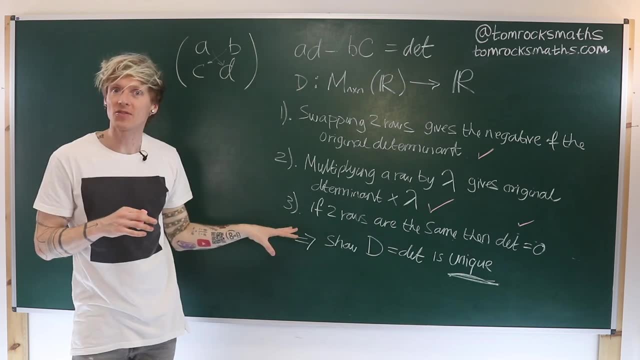 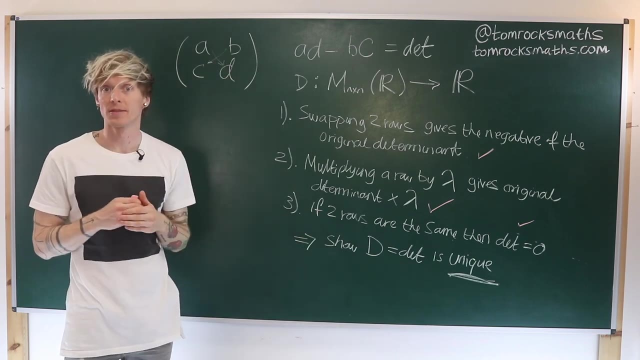 and then we just appeal to uniqueness. So, because we can show any function satisfying these three things, what we have written down here satisfies these three things. therefore, we have found the one and only way of calculating a 2x2 determinant. Don't worry if this all seems a little abstract. 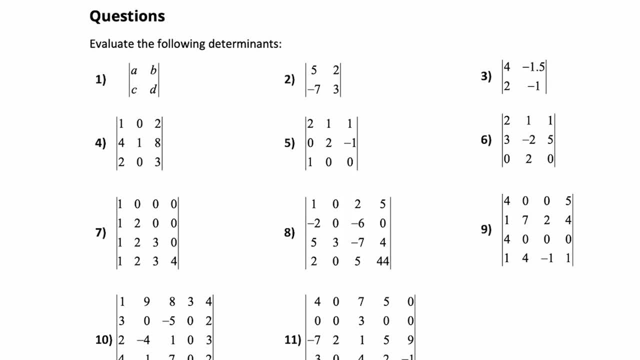 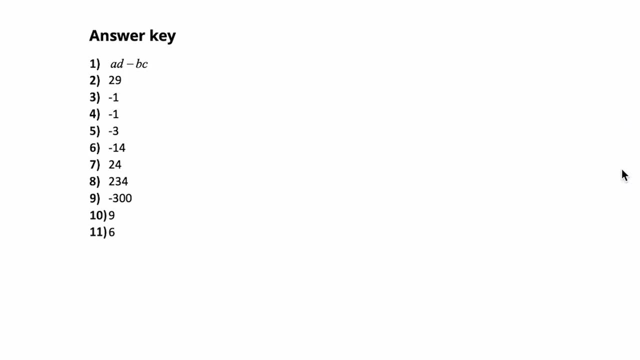 There are plenty of practice exercises, courtesy of ProPrep, which you can access via the links in the video description. There are also answer sheets available so you can check your work and if you sign up for the 30-day free trial. 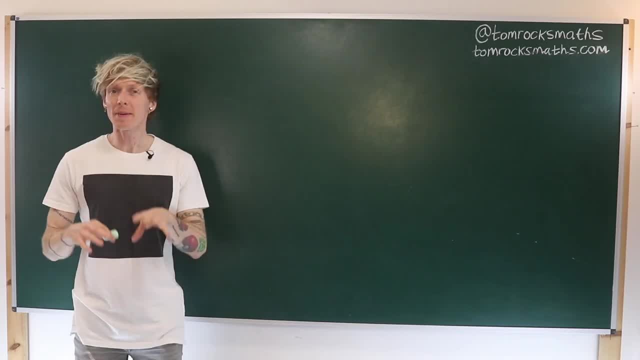 you can watch full video solutions For a 3x3 matrix. the idea is basically the same, except now we have several 2x2 matrices that we need to calculate the determinants of and then combine them in the correct way. 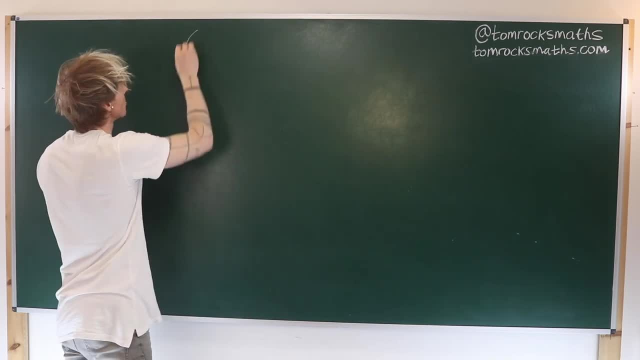 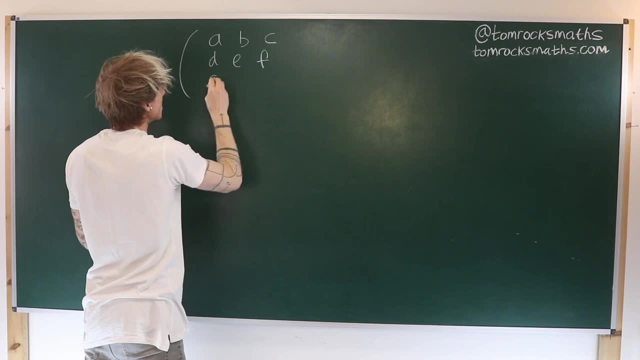 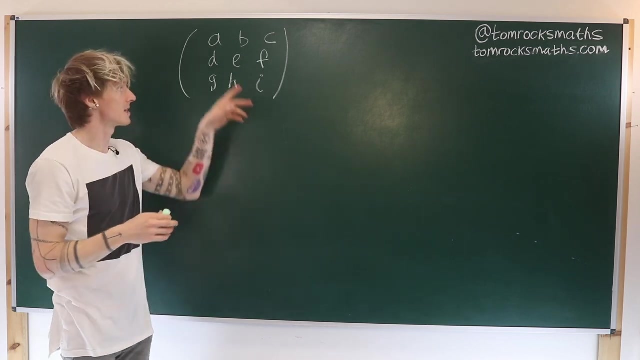 This is how it works, So let's start with a general matrix of a, b, c, d, e, f, g, h, i. So these just represent nine different scalars, nine different real numbers. This is not necessarily e, as in Euler's number. 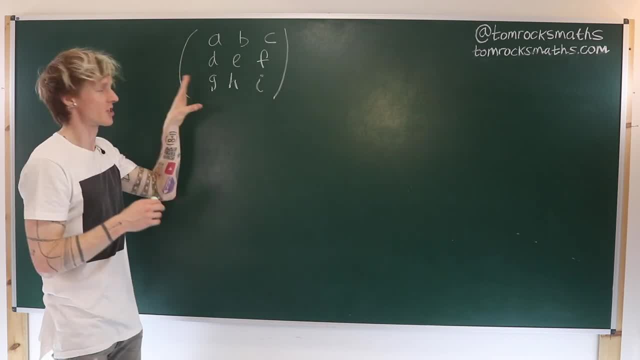 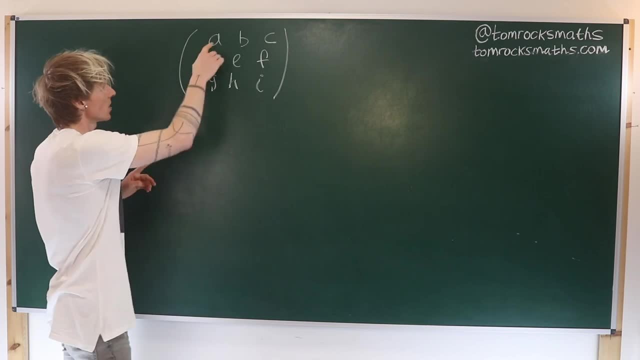 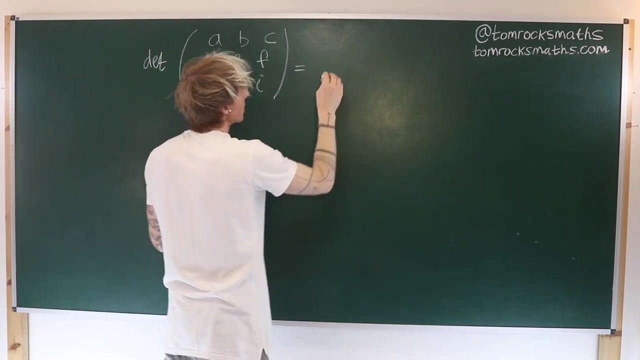 and this is definitely not the square root of minus 1.. These are just nine variables representing the nine entries of our matrix. So we start by taking the first entry, a. so we can say the determinant of this is equal to. We take the first entry, a. 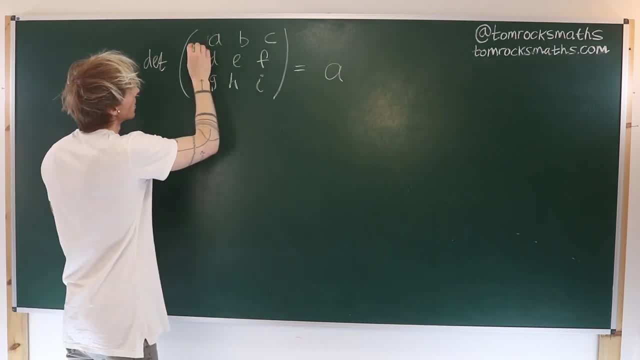 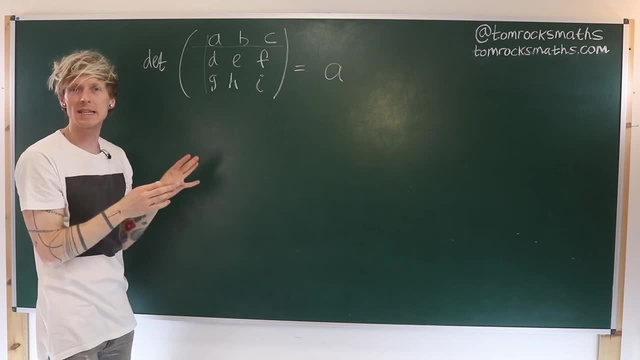 and then we cross off the other entries in that column, the first column and in that first row. So I like to draw these lines in so I can keep track of what I'm doing, because we cross off these rows and this column. 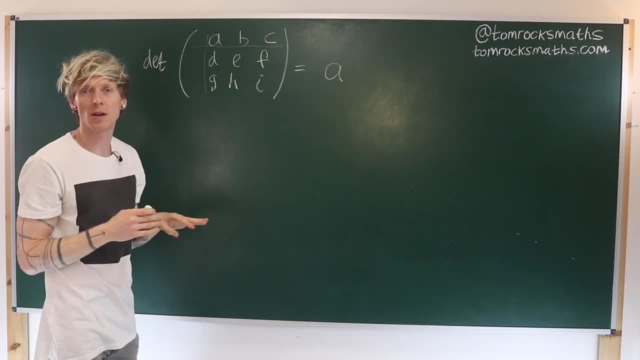 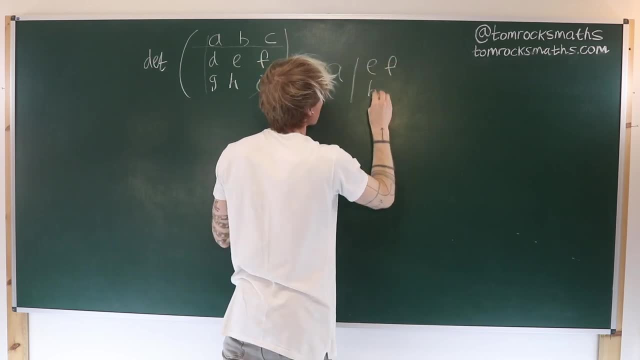 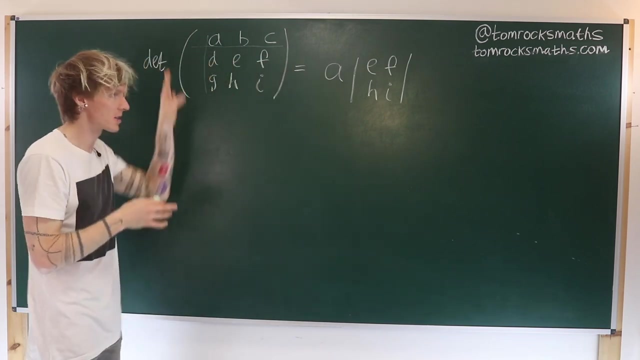 and then we calculate the 2x2 determinant of what's left. So here we're left with the 2x2, which has e, f, h and i. Now that's our first 2x2 that we've calculated as part of the larger calculation. 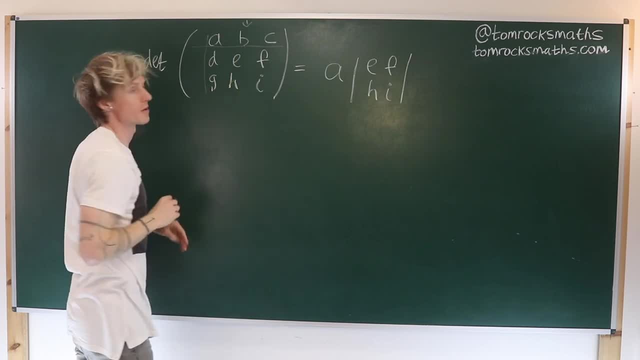 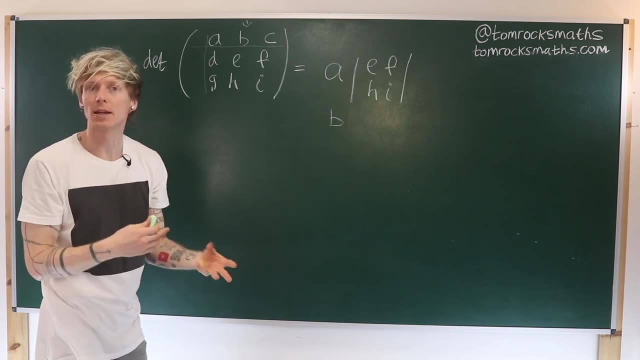 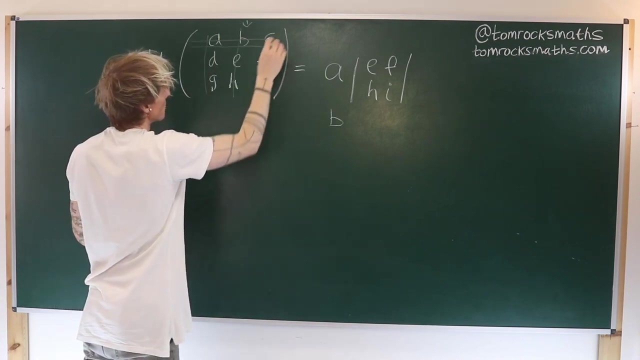 So next we go to this entry here, so b. So we then also have b and we want to multiply by the remaining 2x2 determinant. So for this one we cross off this row and the first column. So you have to think a little bit more about what four entries remain. 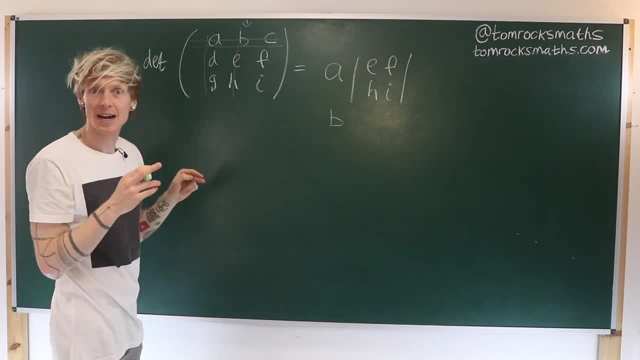 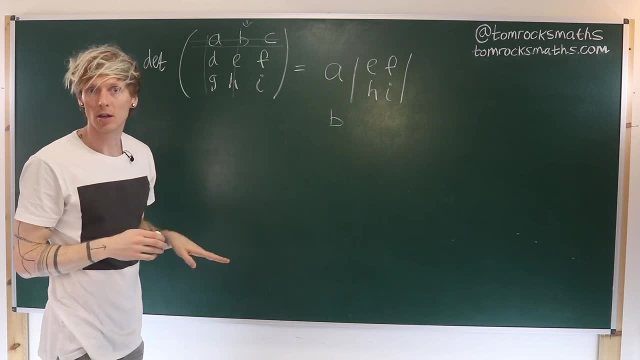 but it's going to be d, g, f and i, because again we cross off the first row and the column that that entry is in. so here the second column. So we're left with a 2x2, which is d, f, g, i. 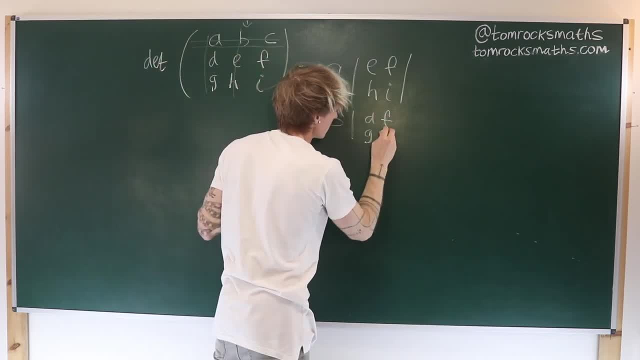 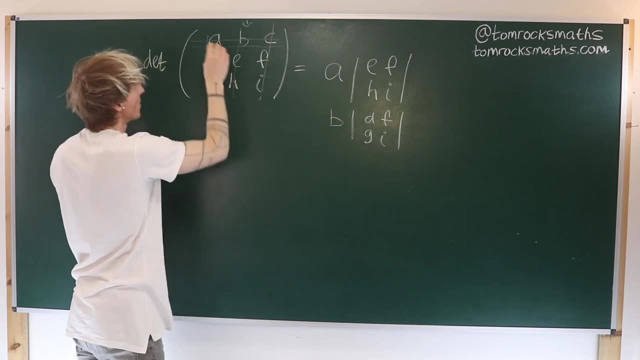 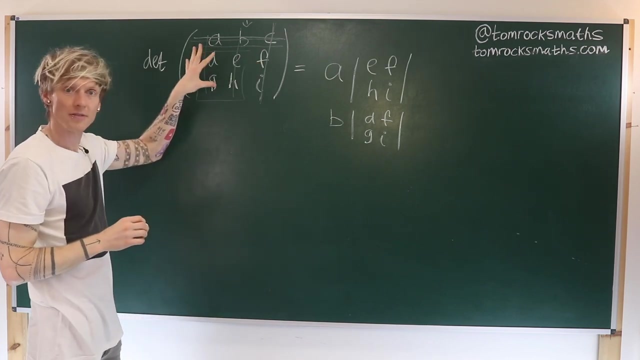 So d, f, g, i, And then finally, we go to the third entry here. so we cross this column off, we cross off the same top row, and what we're going to be left with now is going to be this box here, this lower left corner. 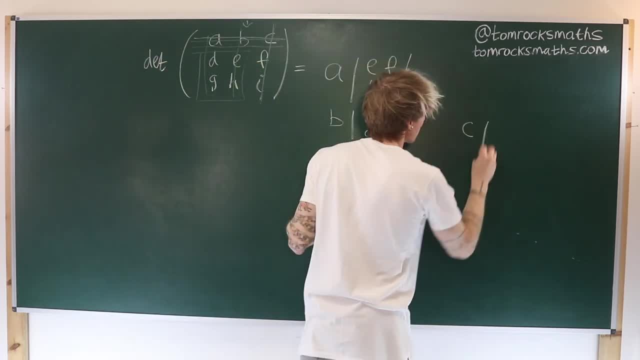 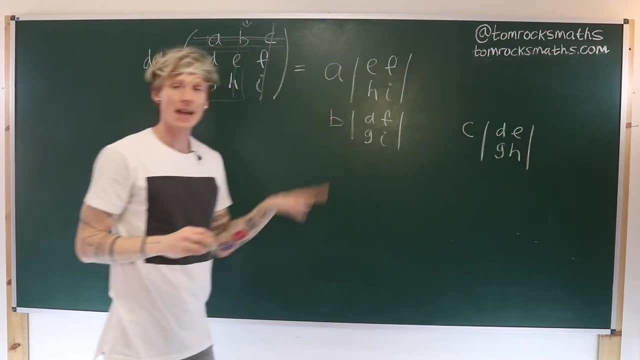 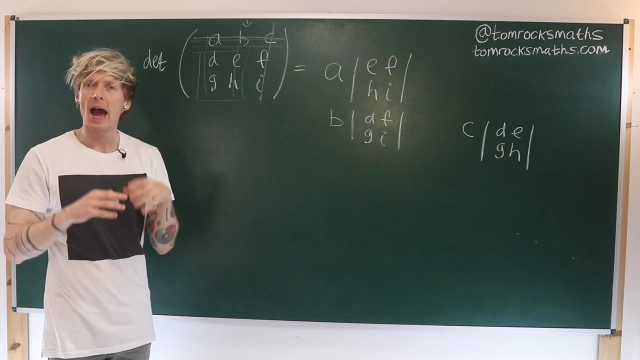 They are the four entries remaining. so we have c times, d, e, g, h. Now we have all of these pieces. the trick is to now combine them in the correct way, And in order to do this, we need to know something called the coefficient matrix. 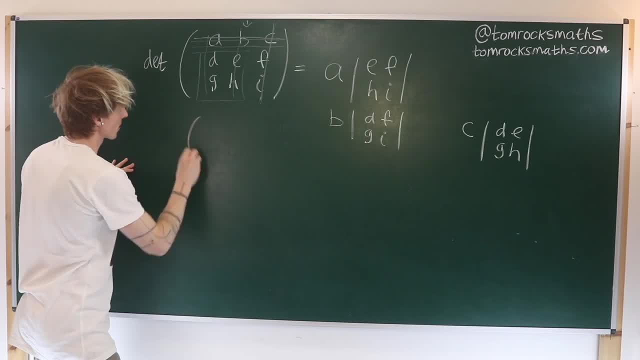 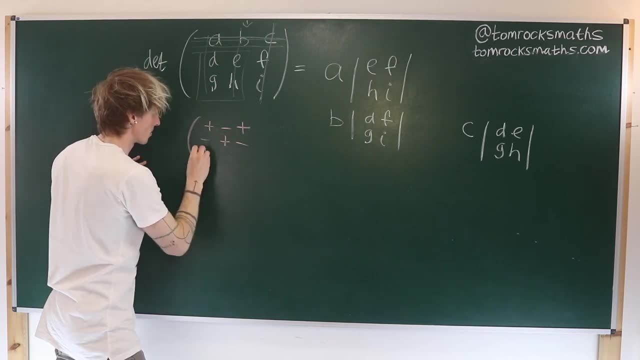 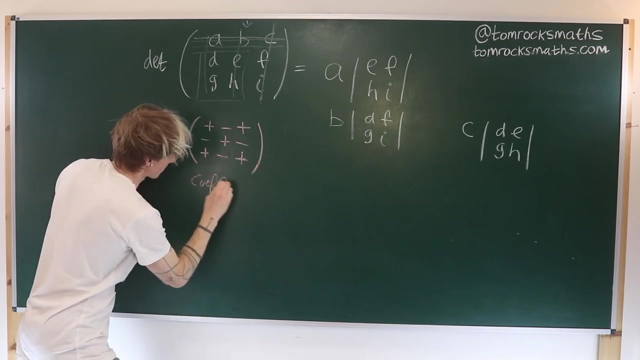 So the coefficient matrix looks like the following: We have, we've got a plus minus plus, then we go back to a minus plus minus and then back to a plus minus plus. So this is our coefficient matrix. 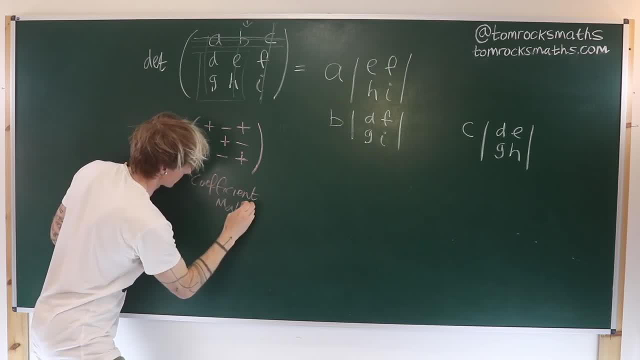 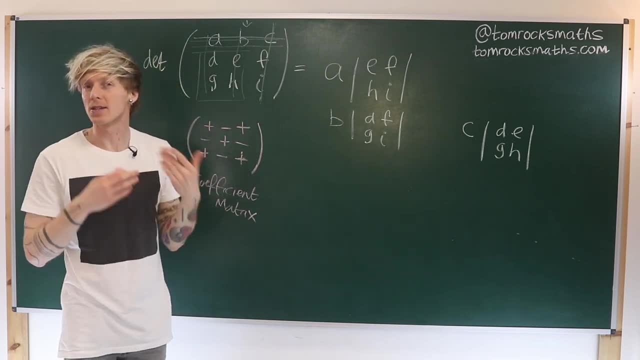 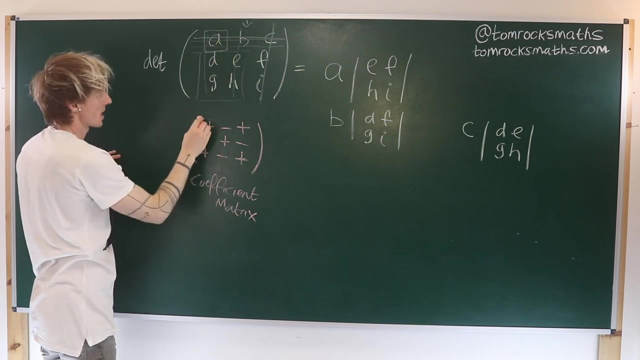 and what this tells us is whether to add or subtract these terms in our 3x3 determinant. So it works as follows: We've got our first entry here, a, and the entry here is a plus, so this is a plus. 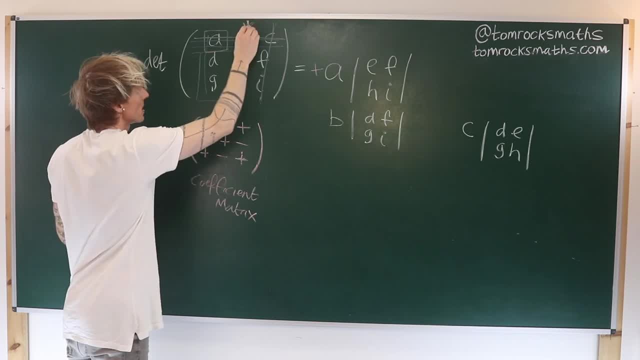 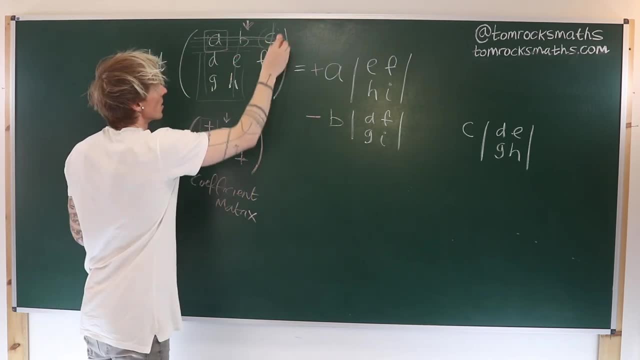 Then we went to the second entry. here we went to b, which is this one here, which is a minus, so we subtract that one. And then again for the third entry, we have c, which is again a plus, so we add this one. 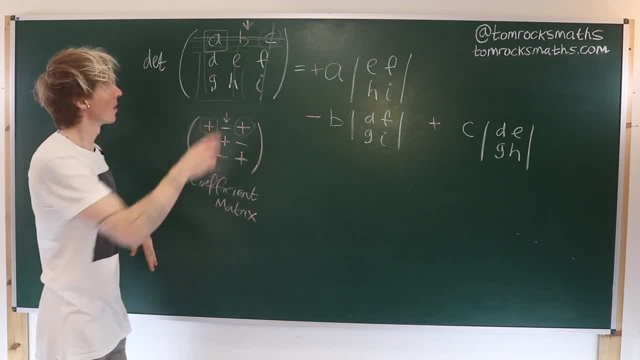 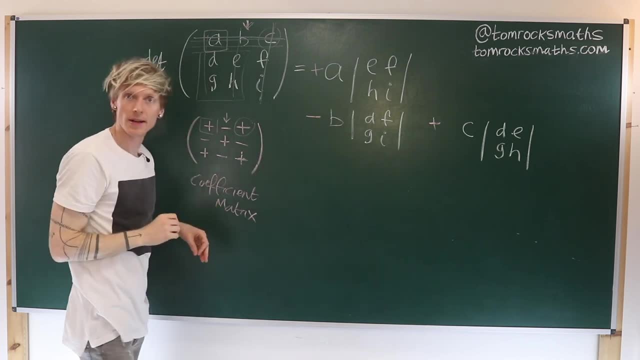 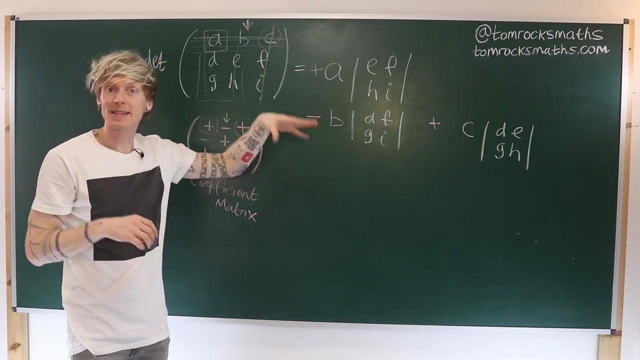 So expanding by the first row as we've done here, we have a times the remaining 2x2 determinant, minus b times the remaining 2x2 determinant and plus c times the remaining 2x2 determinant. Now, of course, we can expand these out. 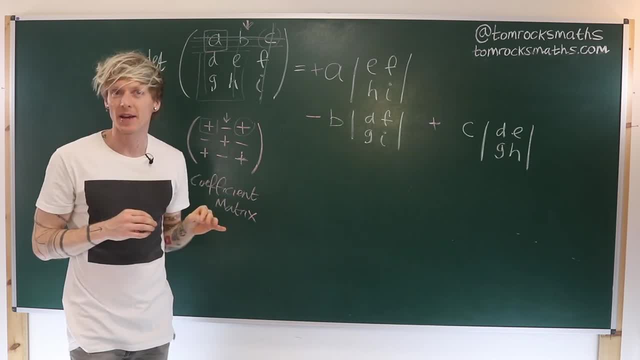 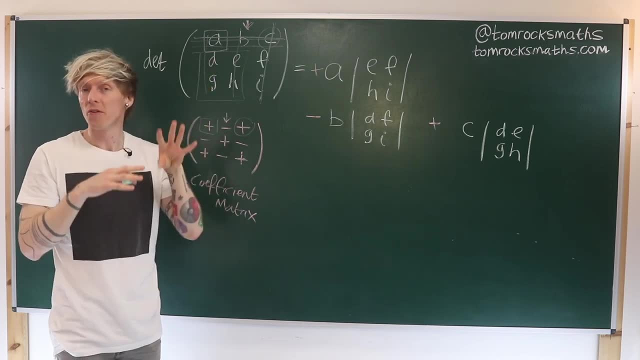 and get the full final answer. so let's do that Using our definition of the 2x2 determinant, which we've just shown is the unique definition for a determinant. we just simply do top left times, bottom right minus the other one. 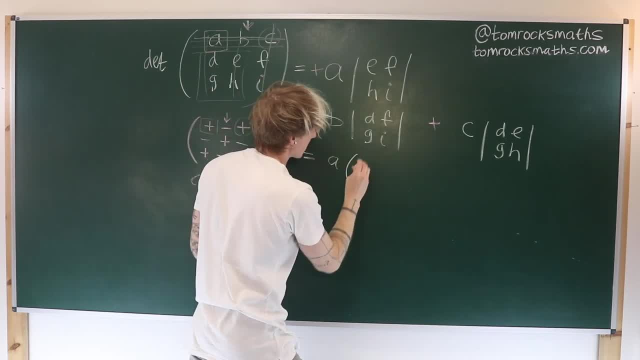 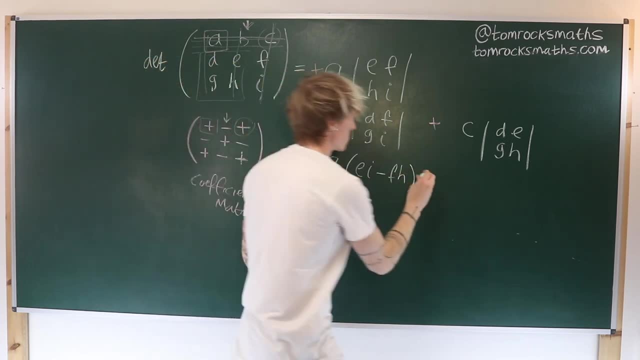 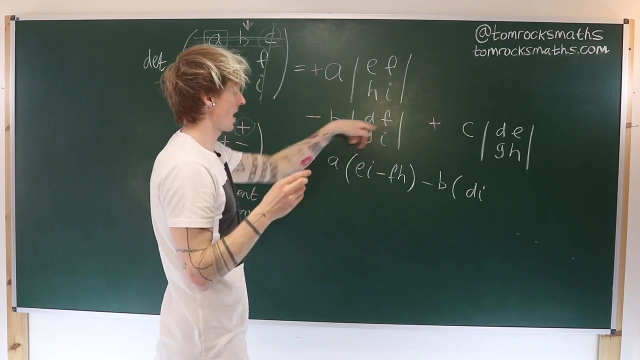 So we're going to get here a times ei minus fh, Then we have minus b times this 2x2, so minus b times di, and then we're going to subtract fg And finally we add on the third one. 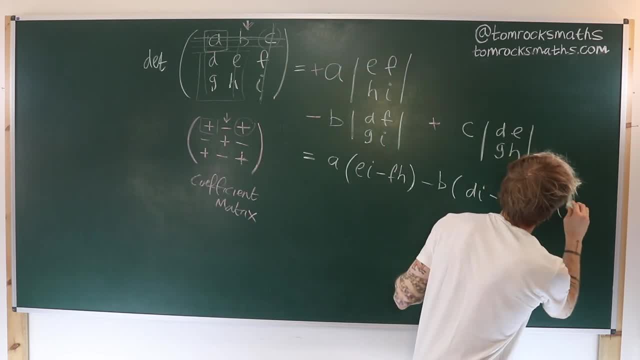 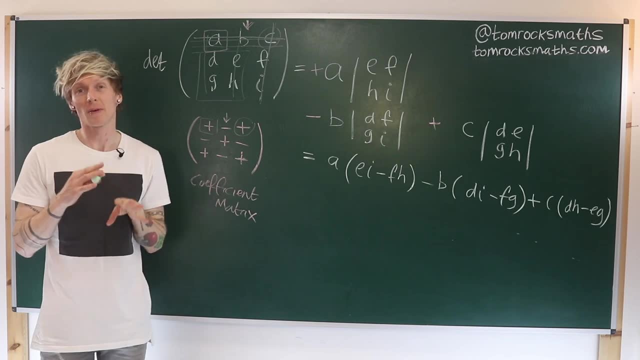 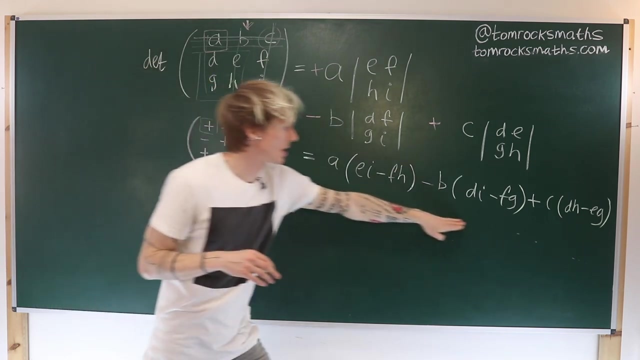 so c, and then it's multiplied by that 2x2, which is dh minus eg. Now, at this stage, there are two important points that I would like to raise. The first one is: given this definition of the determinant: 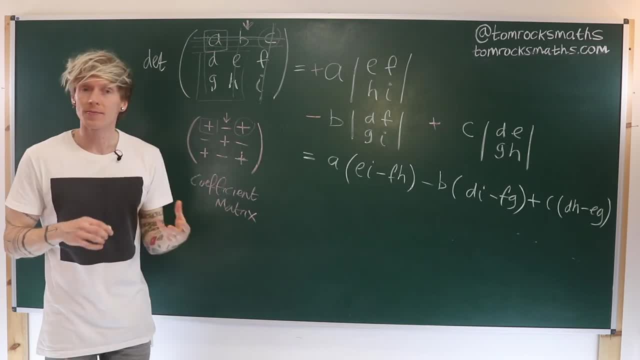 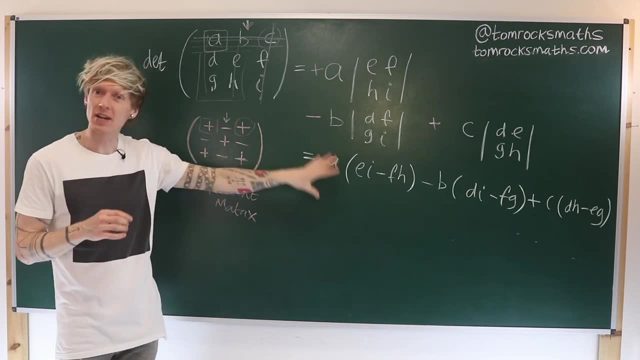 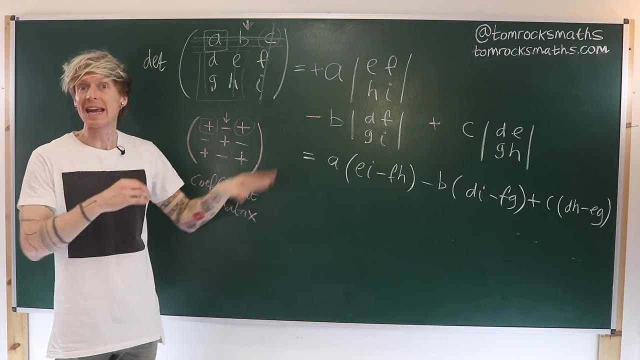 as written here. what you can do is go back to our three determinant properties and you want to check that, using this definition, this formula will satisfy all of those three properties. so therefore, this function is a determinant function for a 3x3 matrix. 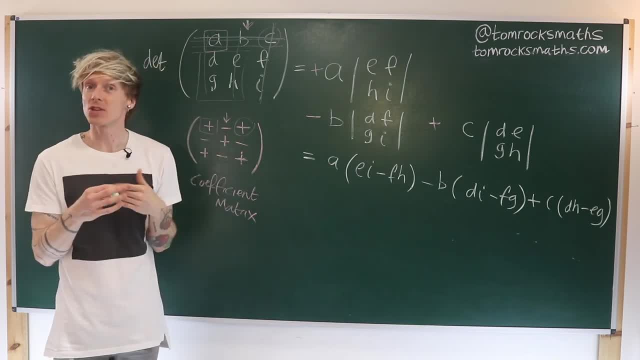 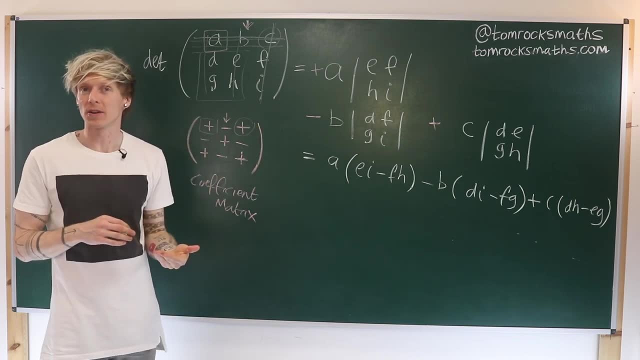 and we can then appeal to uniqueness, just as we did before, to say it's not just a determinant function, it is the determinant function because the uniqueness says there is one and only one such function. So I do recommend, as an exercise to help improve your understanding, 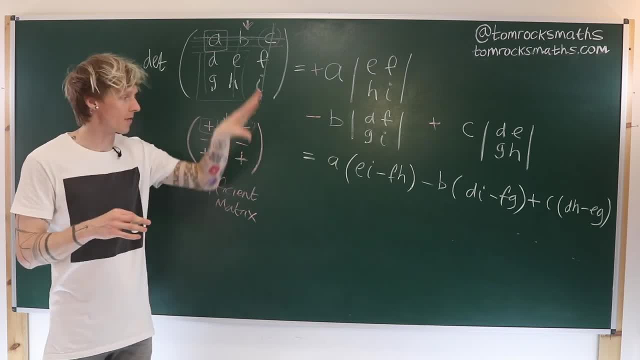 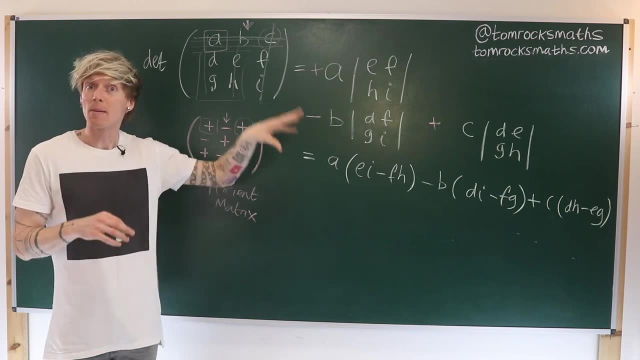 taking this function as our definition of a 3x3 determinant and convince yourself that it does indeed satisfy those three properties that we looked at before. Therefore, this is the one and only determinant for a 3x3 matrix. Now the second point I'd like to discuss here. 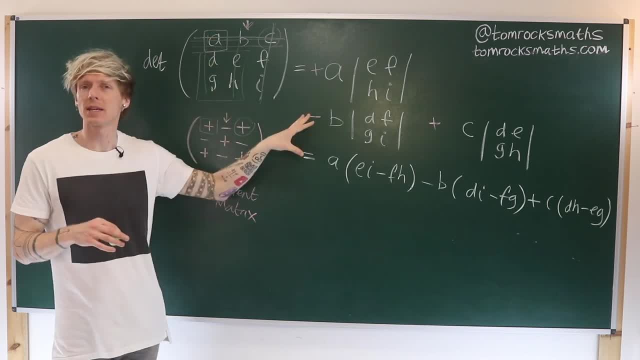 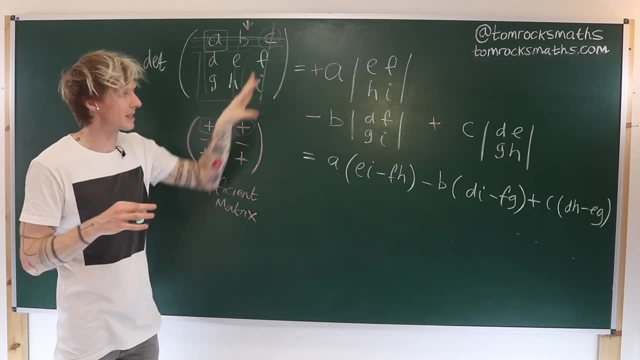 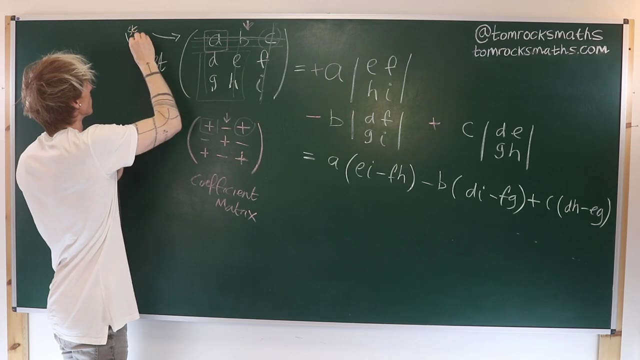 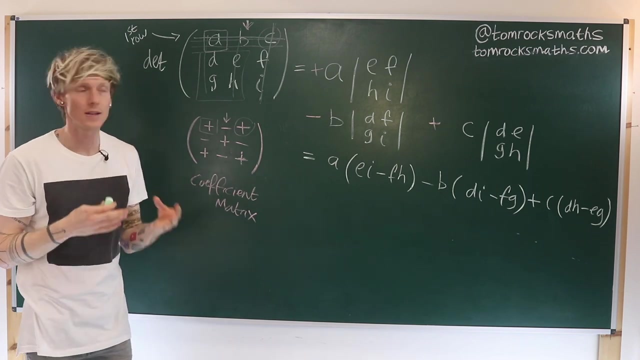 is how we calculated this particular determinant, And what I mean by that is, when I was doing the expansion to get the determinants here, I decided to expand in the first row. Now you don't have to do this. You are, in fact, free to expand in the first row. 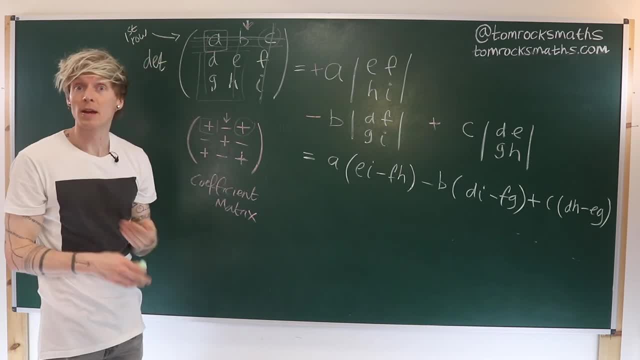 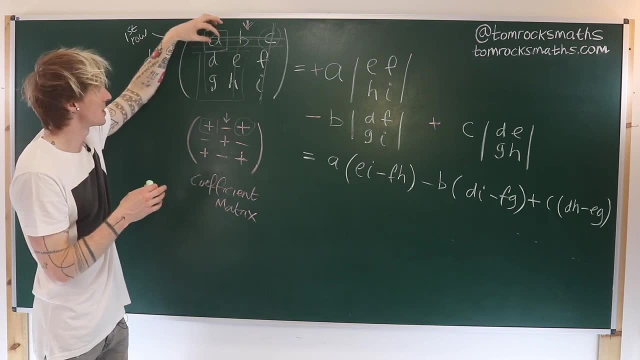 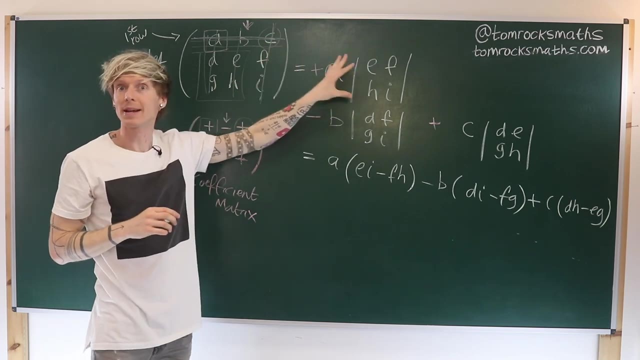 the second row or the third row, remembering that as you expand, you move through the columns and each time you pick an entry, just like we did here with A, you cross off that column and that row and you calculate the remaining 2x2.. 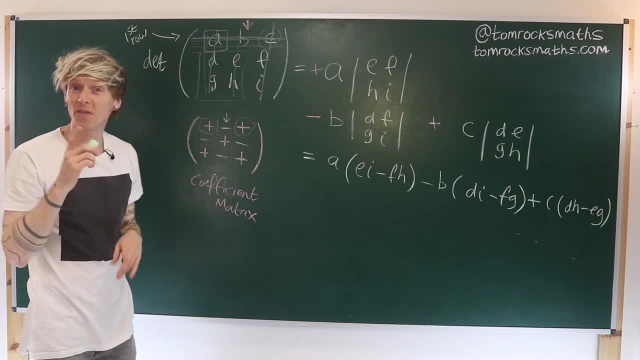 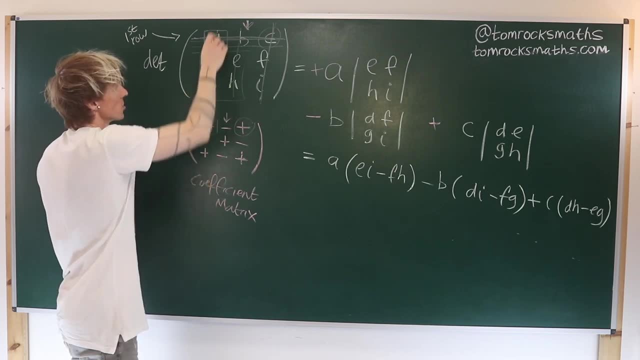 So you can do this for any of the three rows and in fact you can do this for any of the three columns. So again, you could expand down this first column and then you would do A and get the same thing, you'd get D and you'd get that 2x2, BCHI. 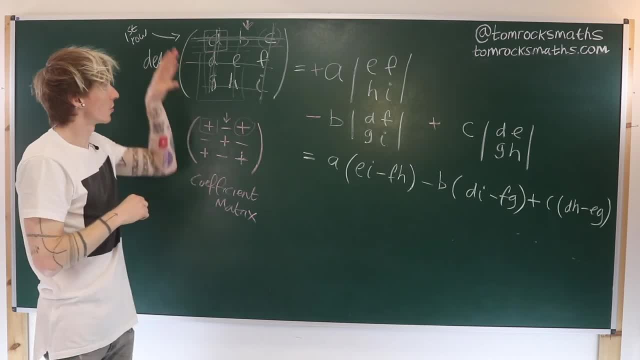 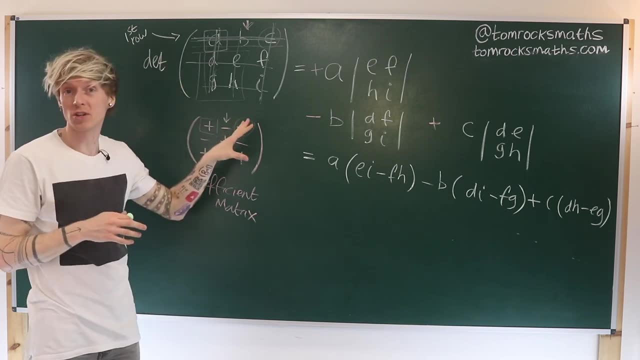 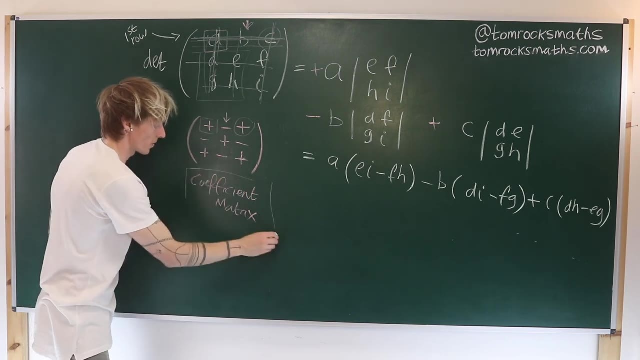 and then you'd get the third one times G. So you're free to expand in any row or any column, And this is actually a really helpful technique, depending on the structure of your matrix. But remember, depending on where you expand, you still have to use the coefficient matrix. 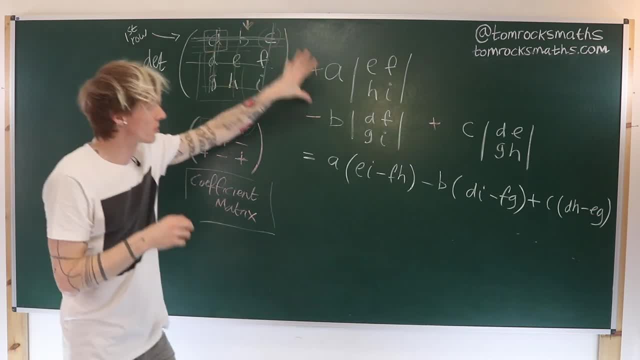 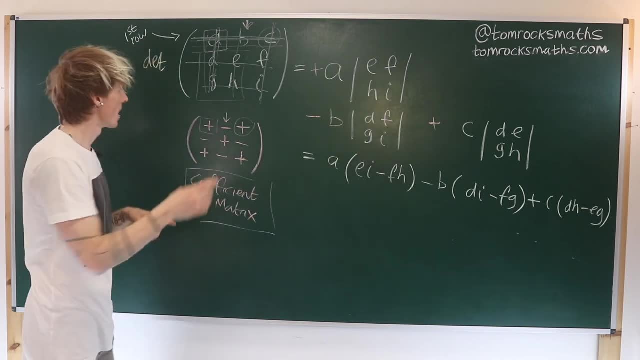 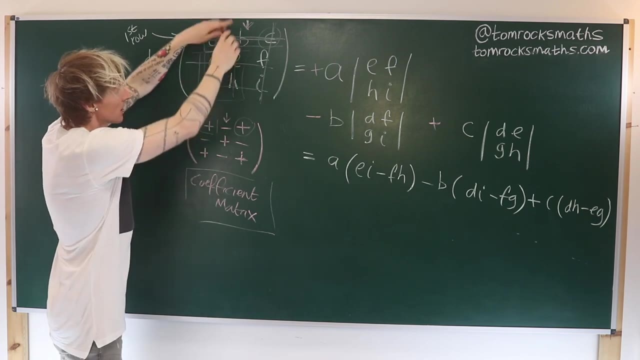 to get the correct signs in front of those three pieces you have in terms of the 2x2 determinants. So, for example, if you expand in the second row, then you have D with a negative, then you add E times the remaining 2x2,. 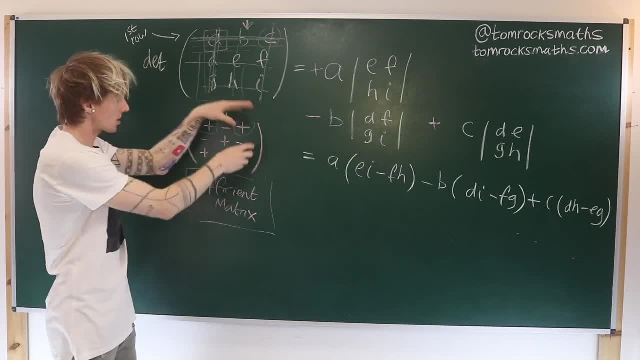 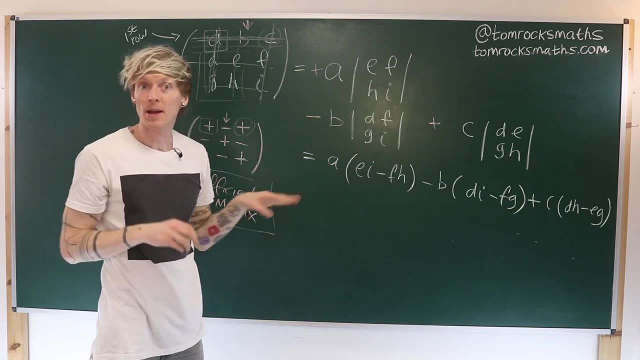 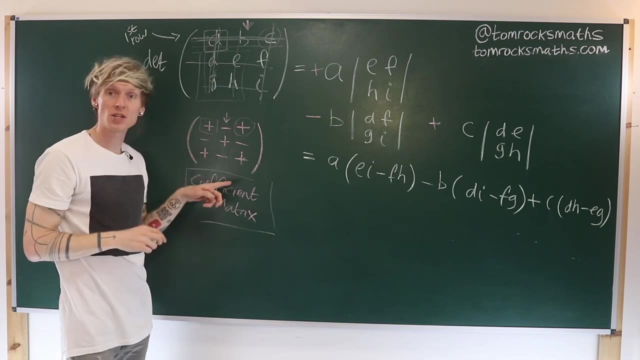 and then you subtract F. So this coefficient matrix is really important, not only in helping you to remember how to expand by the first row, but if you decide to expand by a different row or, in fact, a column, you still need to take the correct coefficient from this matrix. 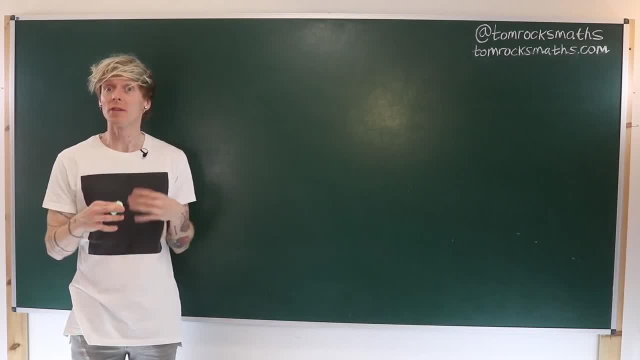 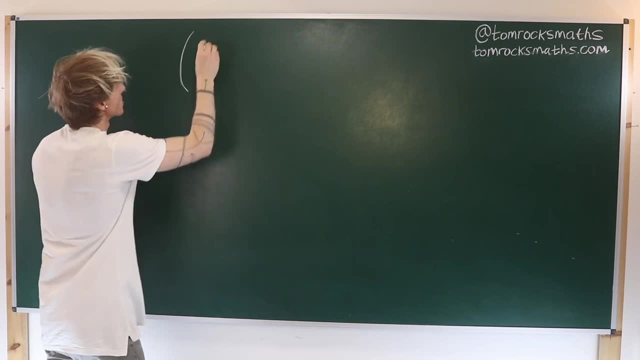 Let's finish by doing an example to see how all of this works in practice. So we're going to consider the following 3x3, matrix. So we'll have 1, 2, 1, minus 5, 10, 1,. 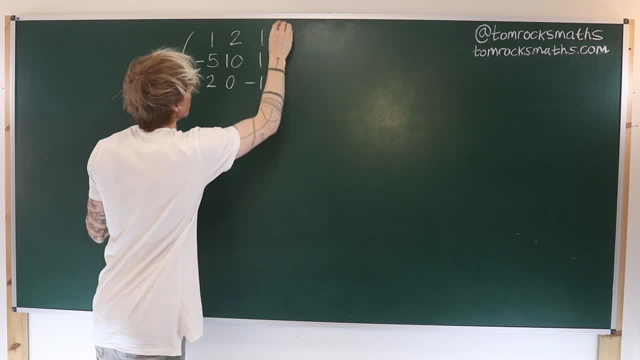 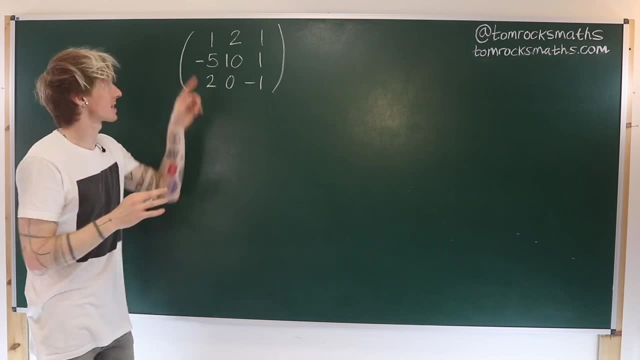 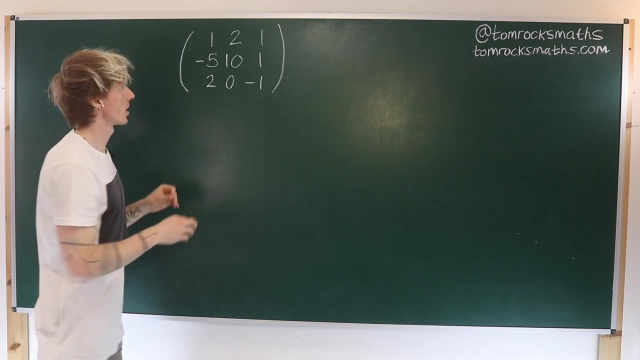 and 2, 0, minus 1.. So a standard 3x3 matrix, all with real entries. So first let's expand using the first row. so this will follow that general formula that we just looked at. So the determinant is equal to. 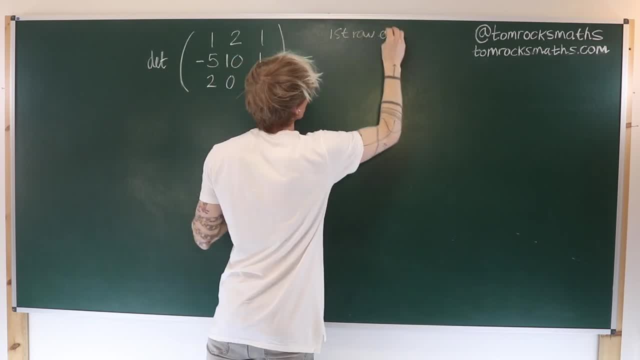 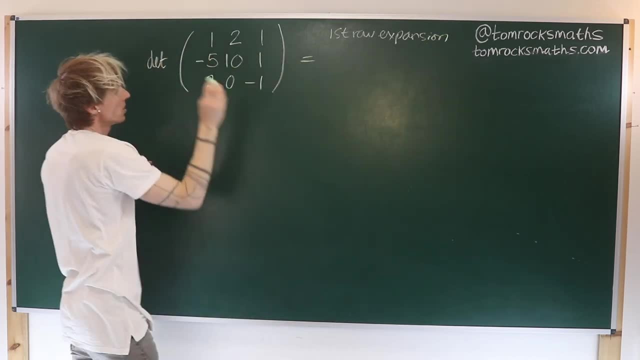 and this is our first row- expansion. Okay, so remember how to do this. We go 1, and it has a plus for our coefficient matrix. So we cross off these and we cross off those, So it's 1 times the remaining 2x2 determinant. 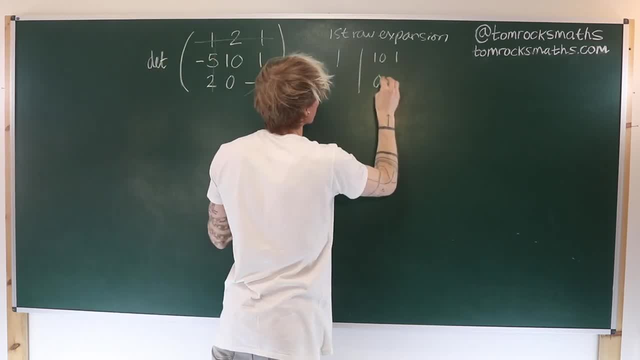 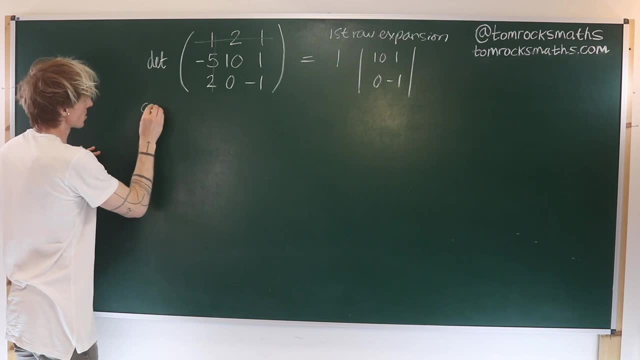 which is 10, 1, 0, minus 1.. 10, 1, 0, minus 1.. Now I do remember what goes next, but let's just check. So the coefficient matrix. always a good idea to write this out, in my opinion. 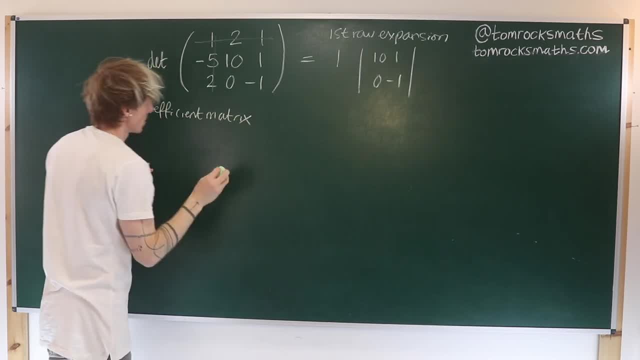 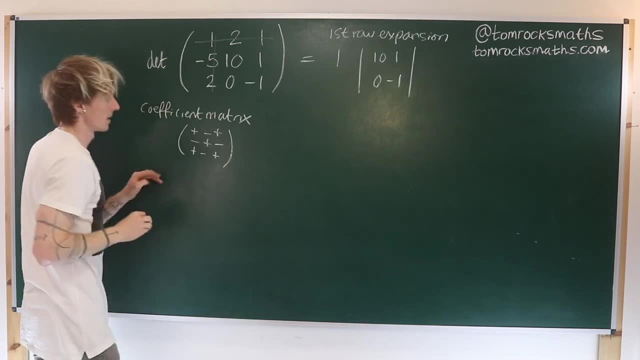 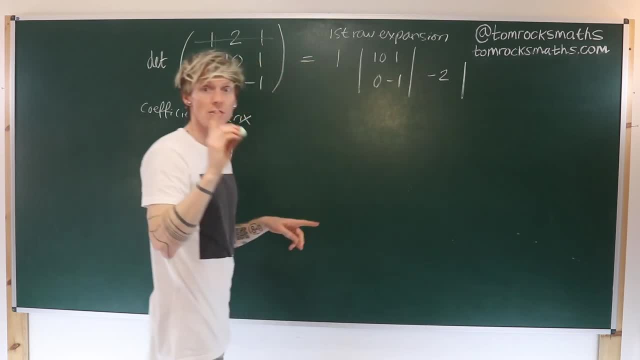 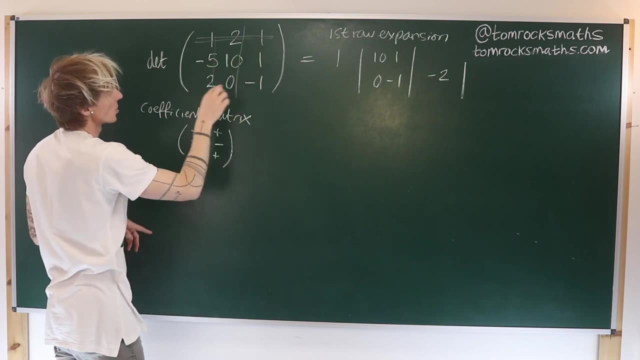 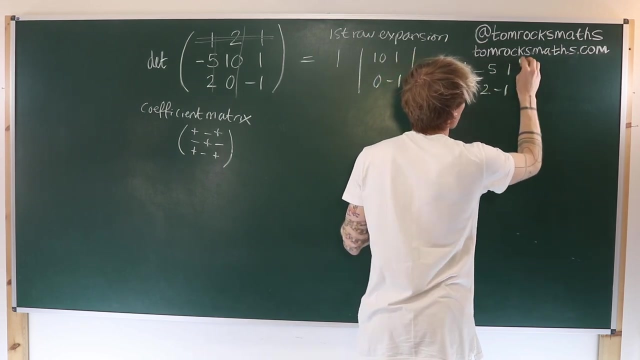 So it's this minus 2, and then the 2x2 determinant that we're left with crossing those off now is going to be minus 5, 1, 2, and minus 1.. So minus 5,, 1, 2, and minus 1.. 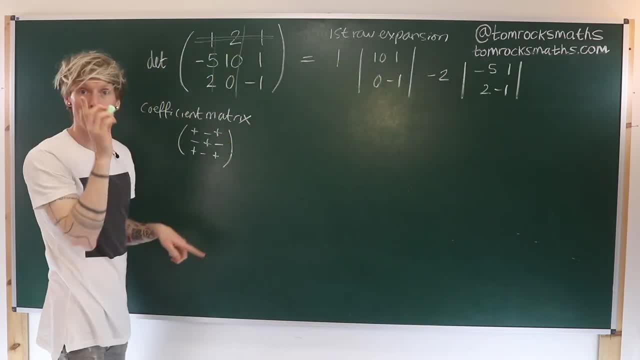 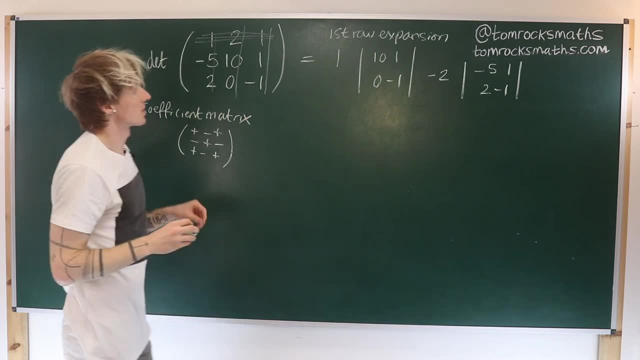 And then the third and final term. so that's now a plus and we have 1, so we cross off this 1 and the top and we're left with these elements. So it's going to now be plus 1,. 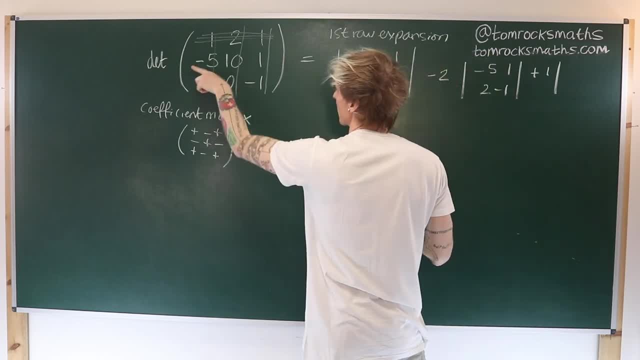 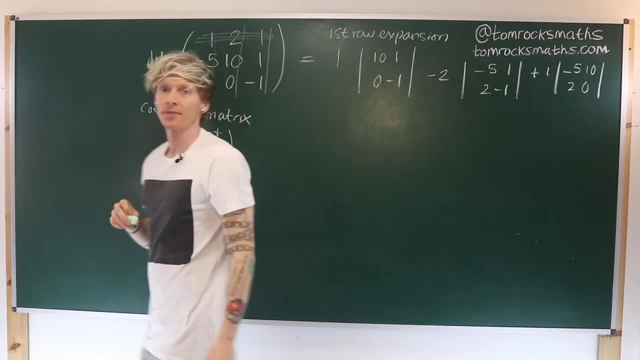 and that's multiplied by this: 2x2, minus 5, 10, minus 5, 10, 2, 0.. Okay, so if we now expand out the 2x2 determinants, we've got 1 multiplied by. 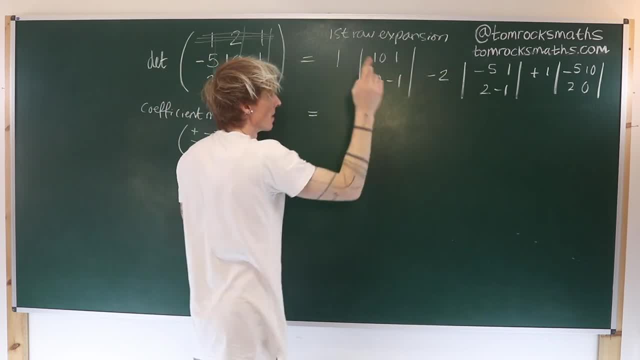 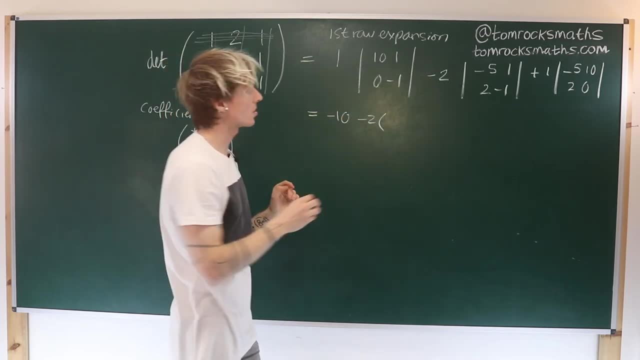 top left, bottom right, minus 10, minus 0. So that's minus 10 in total. Then we have minus 2 times the 2x2, so minus 5 times minus 1 is 5, minus 2, so that gives you 3,. 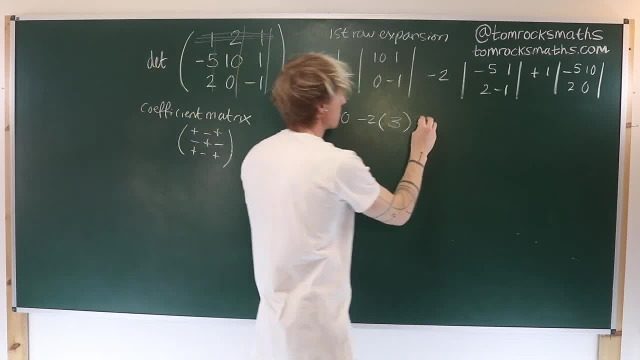 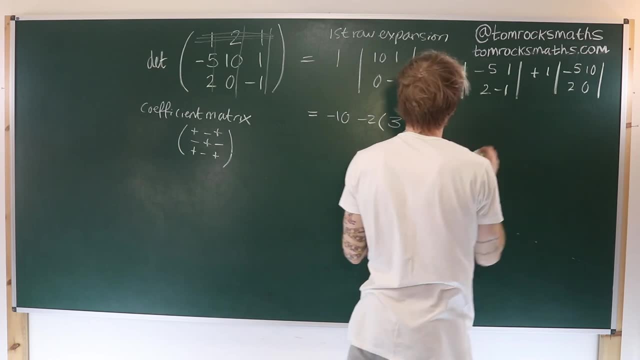 for that 2x2 determinant. And then we've got plus 1 multiplied by that determinant. so minus 5 times 0 is 0, minus 20.. So it's plus 1 lot of minus 20.. So putting this all together, 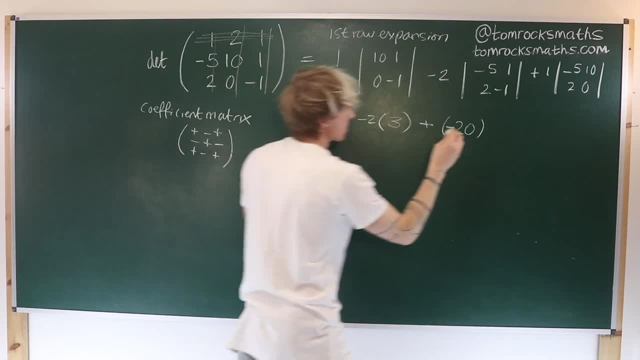 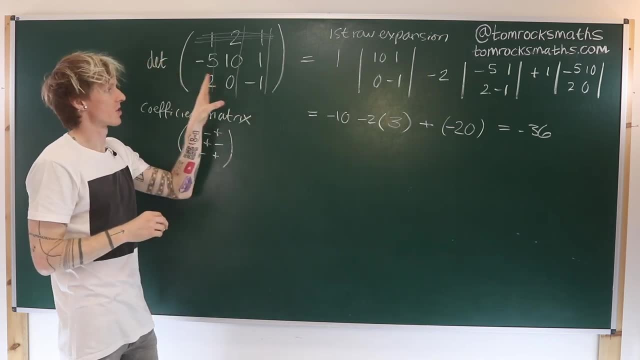 we've got minus 10,, minus another 6,, minus 20,, so that equals minus 36.. So the determinant of this matrix, this 3x3 matrix, using the general formula and expanding in row 1, gives us minus 36.. 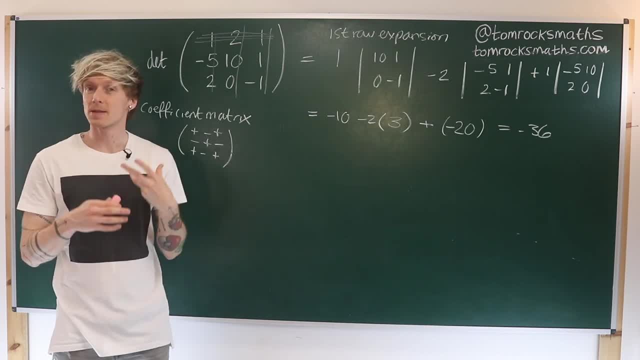 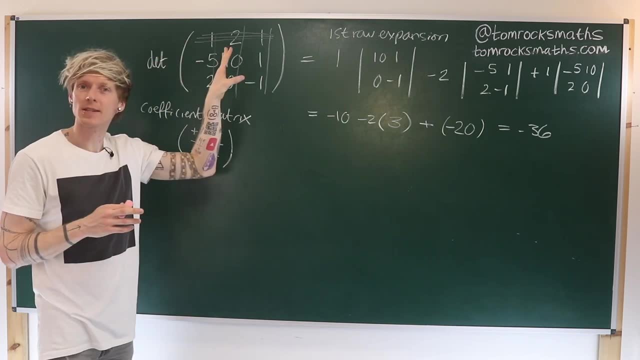 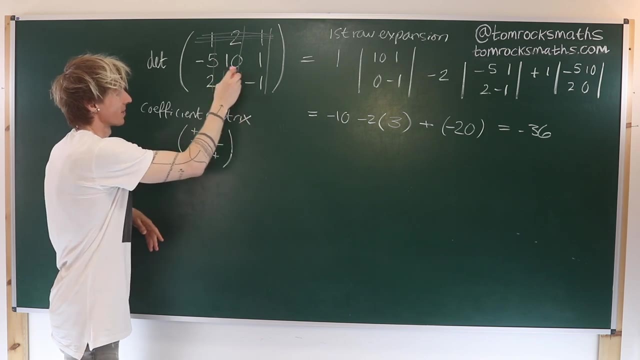 Now remember, I said that you can, in fact, expand via any row or any column. So, looking at our original matrix, where do you think we might want to expand? We have a 0 entry here. Now a 0 entry is going to be really helpful. 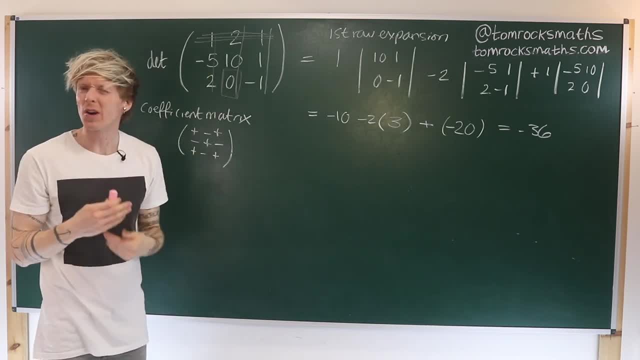 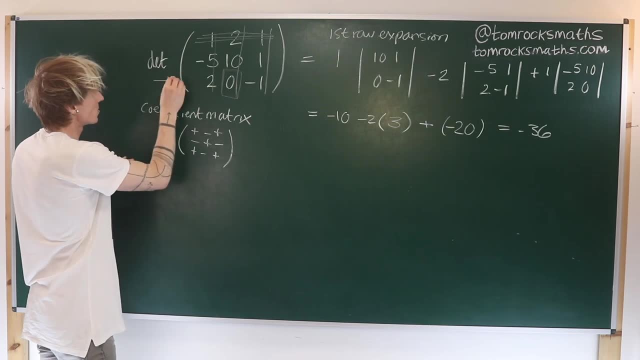 if we have that in our row or in our column, Because when we expand, for example, if we do the third row- which is what we're going to do when you do the third row- that second group term, that second term multiplied by a 2x2,. 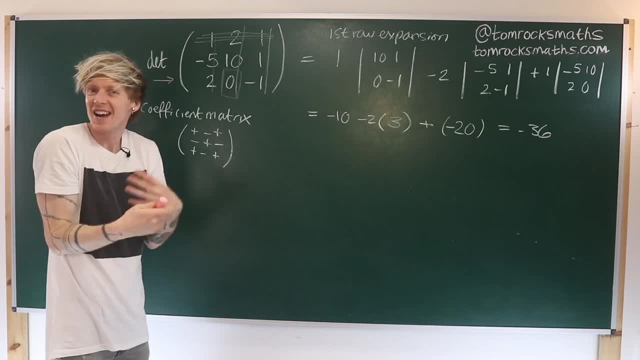 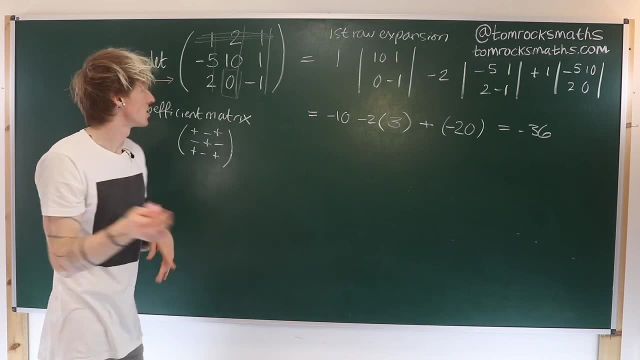 it's 0 times the 2x2.. So we don't actually need to calculate the 2x2, because it's going to be multiplied by 0, and therefore always give us 0.. So expanding here, expanding in the third row. 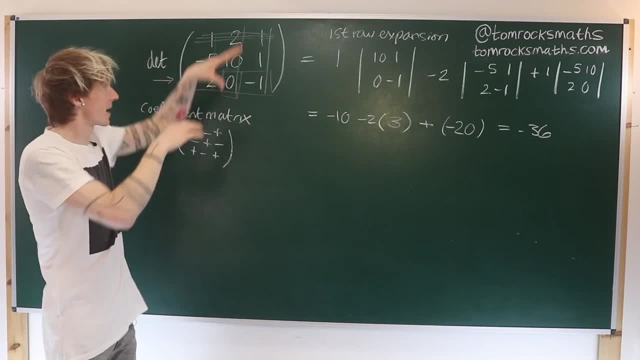 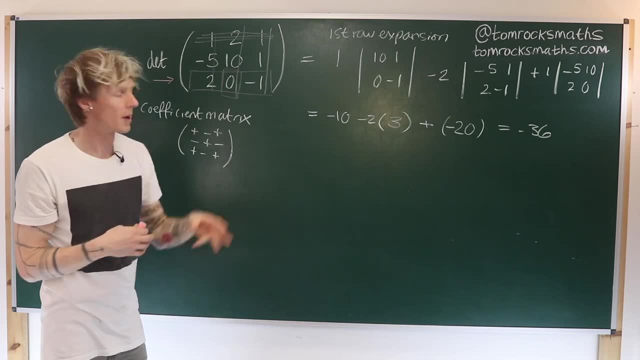 is actually going to save us some work. So if I had really thought about the best approach to tackle this question, it's always going to be expanding the row or column that has the most 0s, So let's now do that expansion in the third row. 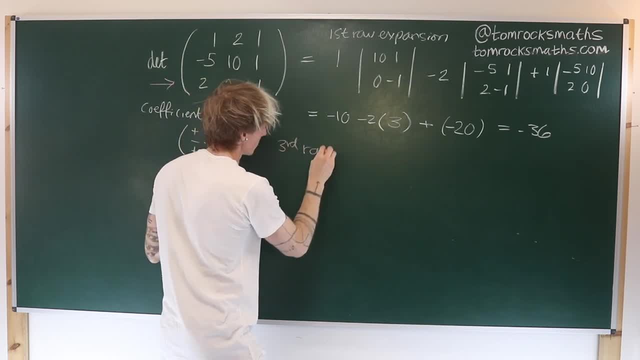 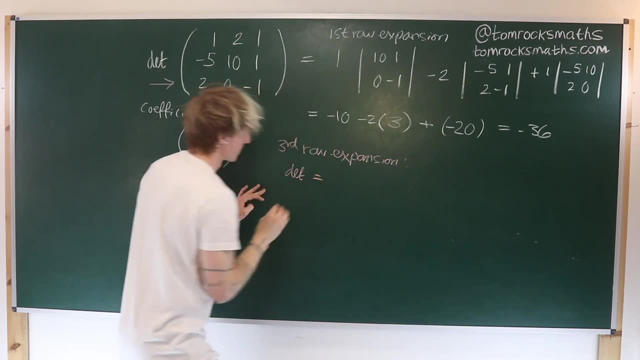 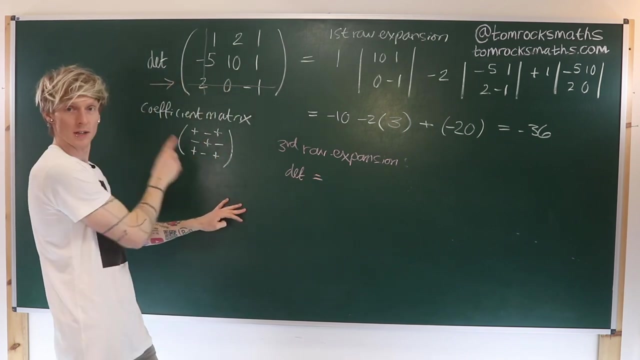 So the third row expansion, the determinant is equal to: we take our first entry, the 2,, and we cross off So we get, and it's a plus from our coefficient matrix. so it's 2 times what's left. 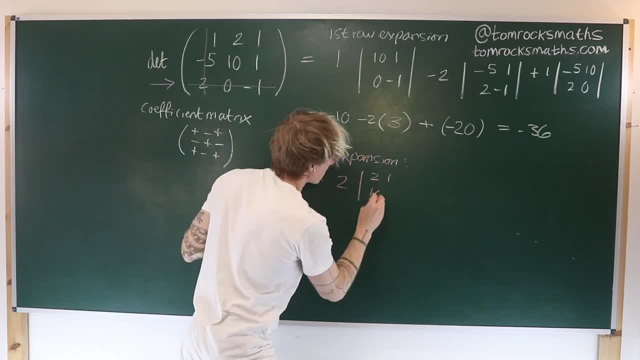 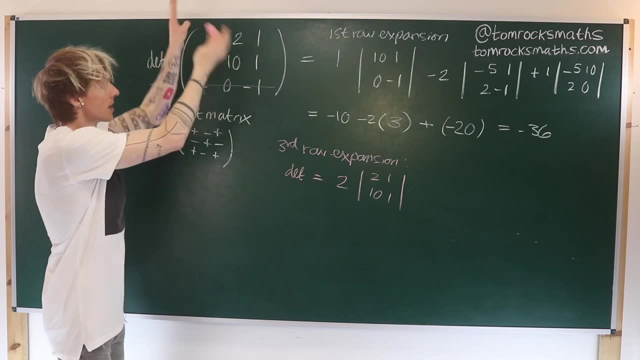 which is 2, 1, 10, 1.. 2, 1, 10, 1.. Then we've got 0, so minus 0 times a 2x2.. But it doesn't actually matter what that 2x2 determinant is. 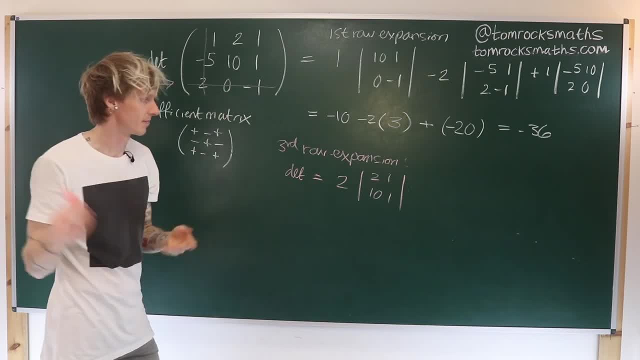 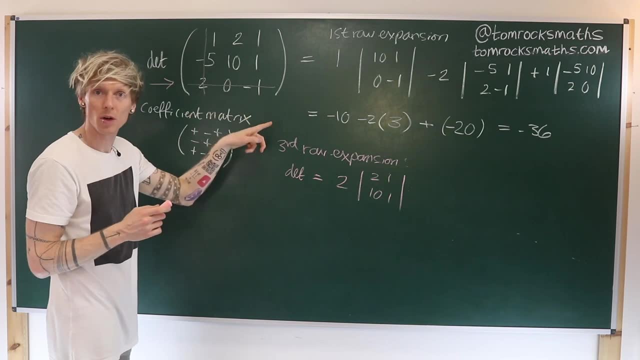 because it's being multiplied by 0, so we get 0.. So we have nothing for that next term. And then the final term is: again it's a plus and we've got a minus 1.. So plus minus 1 gives us a minus. 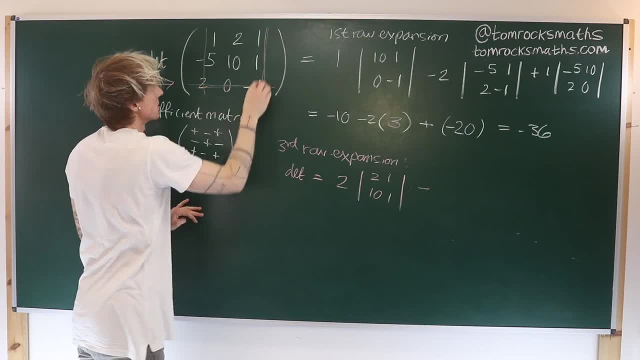 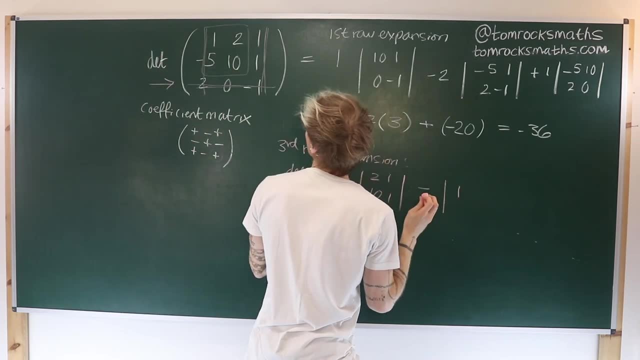 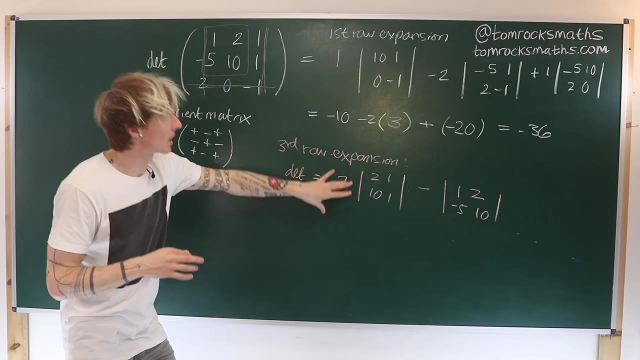 times the 2x2 that's left, which is going to be this section top left section up here. So minus the determinant of 1, 2, minus 5, 10.. So you can already see that this looks a lot simpler. 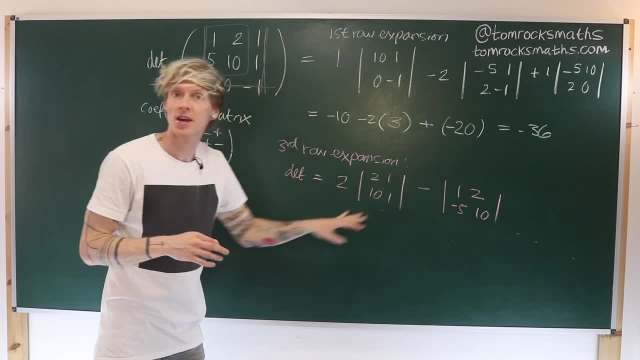 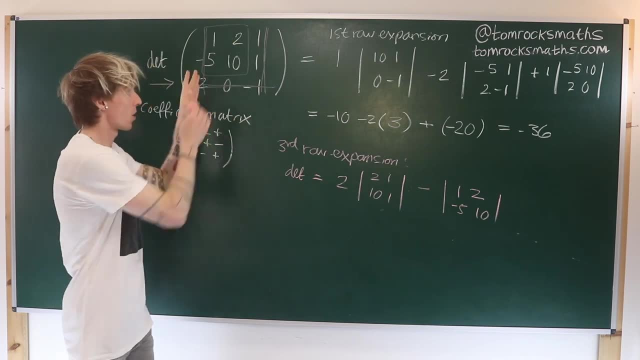 than what we had at the top of the board, because we only have two lots of 2x2 determinants to calculate compared to 3. And this is how this clever choice of where to expand, where we have those zeros, can actually be really helpful. 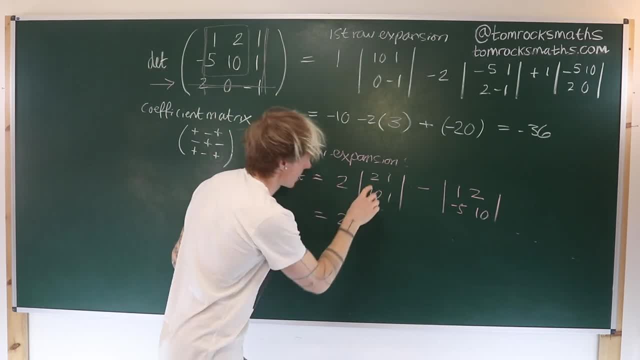 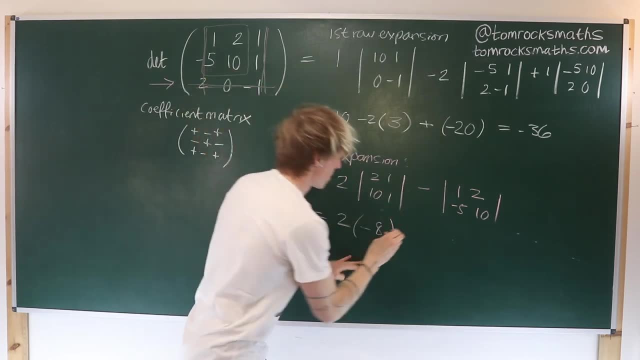 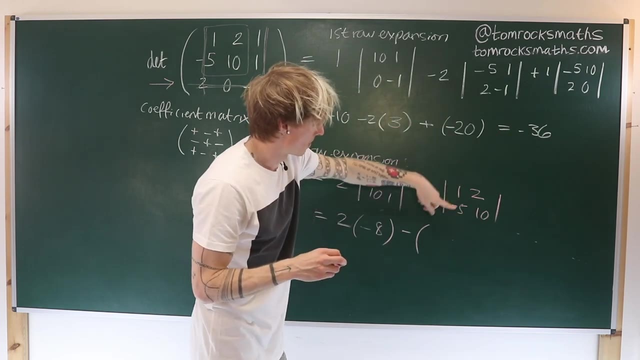 So, doing these expansions, we have 2 times. the determinant is 2 minus 10, so that's minus 8.. And then we've got minus. now for this determinant, we've got 10 minus minus 5 times 2..